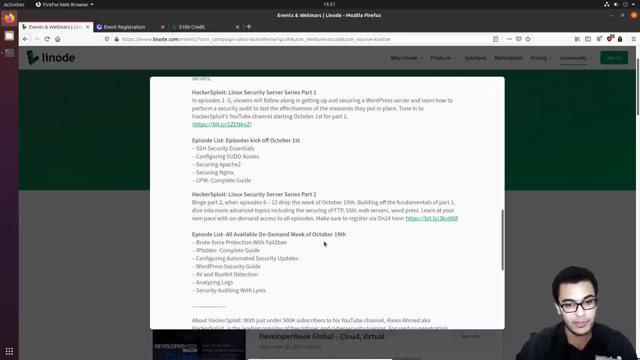 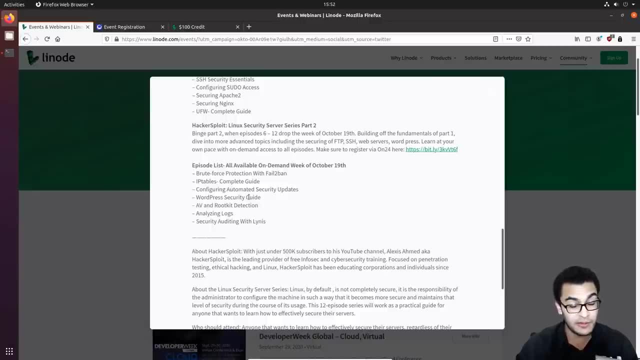 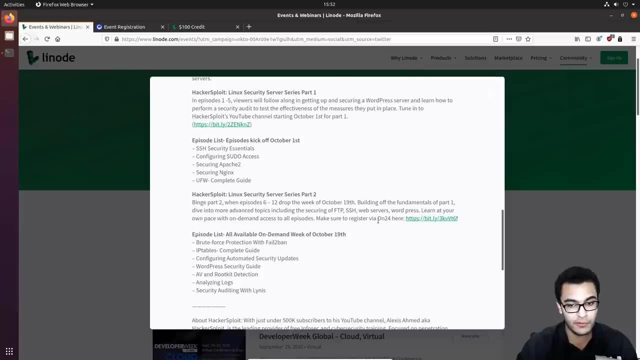 there. This is going to be an advanced series that will build up or build off the first series, And we'll cover things like brute force protection, IP tables, WordPress security and security auditing on Linux with the Linus tool. So to access that, just click on the registration link on the ON24 platform. 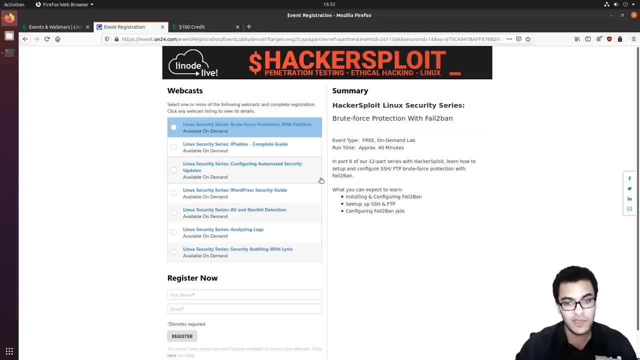 And that'll take you here, So that'll give you an idea of all the various webcasts and when they're going to be posted And it'll give you a summary of what will be covered exactly. These are advanced webcasts that will be about 40 minutes. 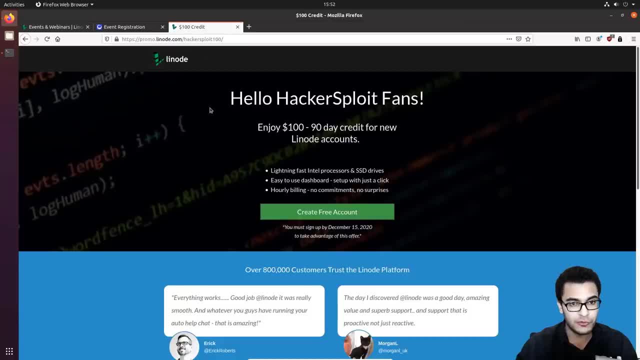 And you can register for them absolutely free of charge. We've also partnered with Linode to give you guys a free credit. So again, if you are interested in using Linode for your virtual private server or for your hosting- whether you're a developer or a administrator- you can get $100. of 90 day credit, And this is for new accounts, So that's fantastic. Definitely do take advantage of this. if you're getting started with Linux or you're actually following, you're following along with this series. You actually redeem this offer or this code, which is under promolinodecom, And the code is: 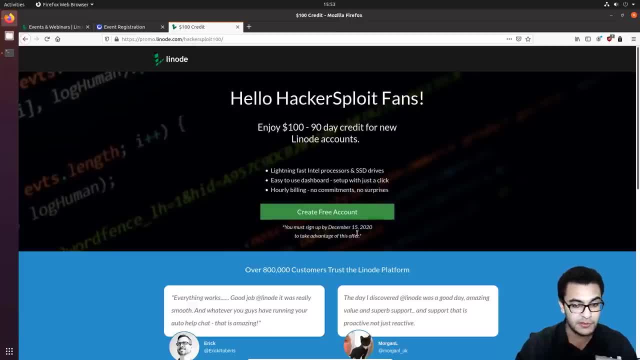 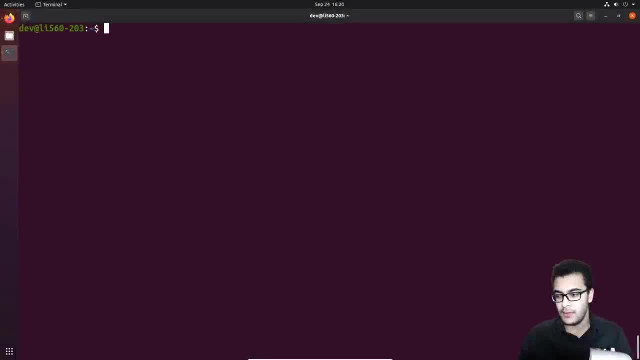 Hackersploit100.. This offer will only be limited till the 15th of December, So definitely check that out. That being said, let's get started with today's video. Hey guys, Hackersploit here back again with another video. Welcome back to the Linux security series. 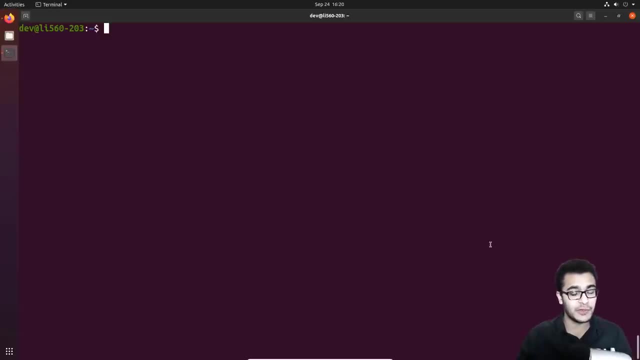 In this video, we're going to be taking a look at how to set up and configure the uncomplicated firewall rules also known as UFW. Alright, so let me just give you a bit of a background as to what UFW is and how it works and its relation with with IP tables. Now, UFW is a utility that is designed 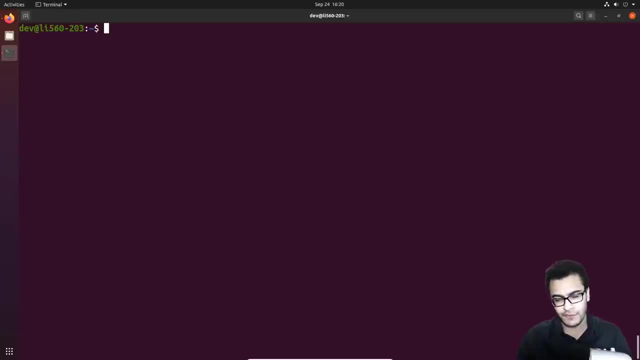 to simplify the setup and management of firewall rules in more specific, IP tables rules. Now, when I say that, essentially, UFW allows you to very easily and very succinctly control, set up your various firewall rules, And the main utility or the tool that UFW uses to do this is IP tables right, So we can actually get. 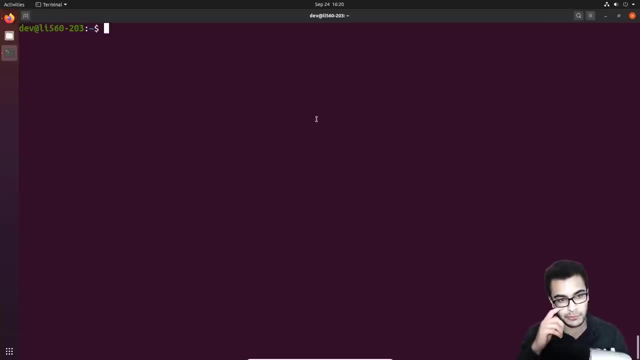 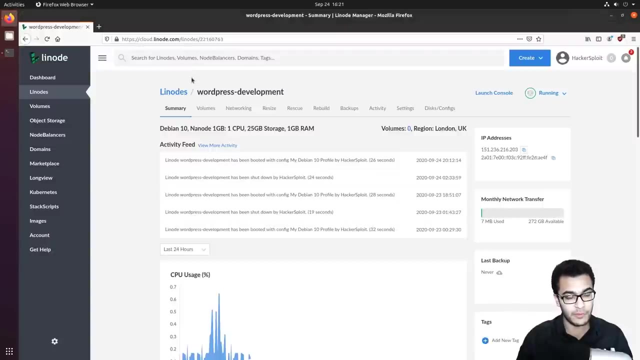 started immediately with it. As mentioned, we're going to be following the example we had set up in the beginning, So our job is to secure the development server that's currently running WordPress, And we're now within the stages of setting up a firewall. And again, we're going to 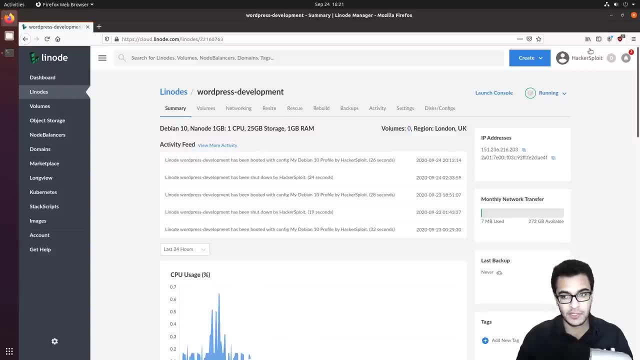 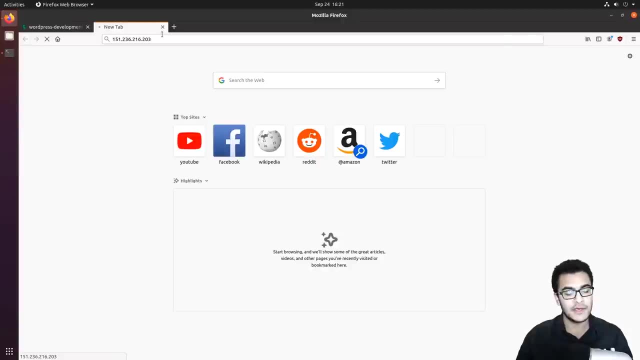 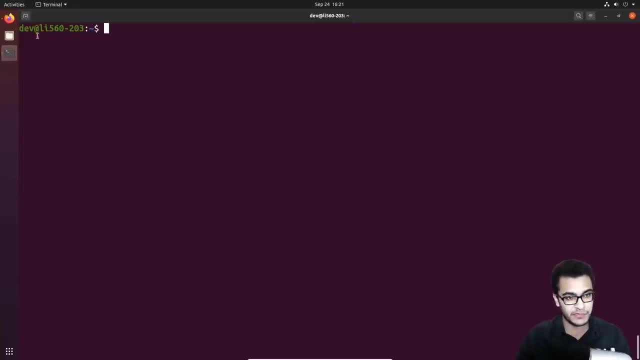 be using a UFW. So right over here we have, if we try and access the web server, we can see that we can pretty much access any service on the target that's currently running. So in this case we have the website running on port 80. And of course, I've been able to establish access using 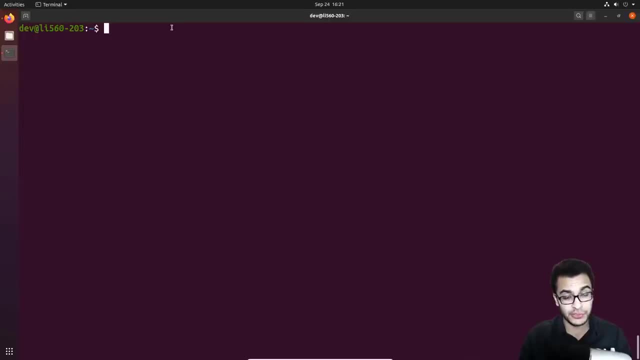 SSH. So the first thing we want to do is we want to ensure that we have UFW installed Now. by default, UFW comes pre-packaged and installed with on Debian based distributions, if I'm not mistaken, more specifically, Ubuntu. Now, given that we are using Debian, we can, or we can, confirm that we. 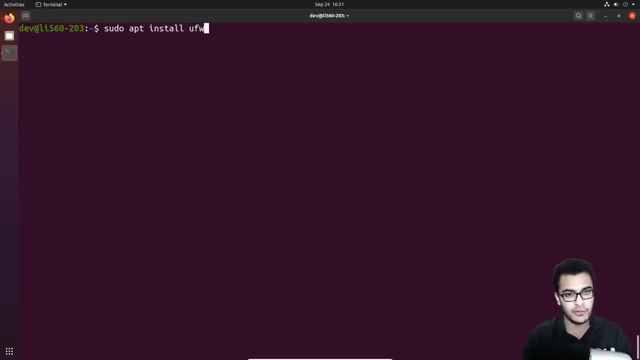 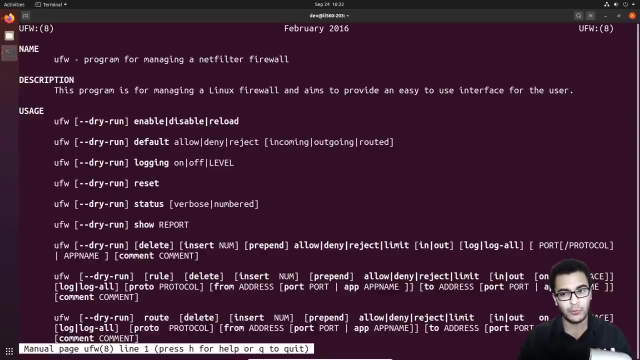 have it installed by saying sudo apt install UFW and we hit enter. I'll just put in the password here And you can see UFW is already the latest version. Of course you can view the UFW manpages to get a bit more of a context as to what this tool is and what it's used for. So again, 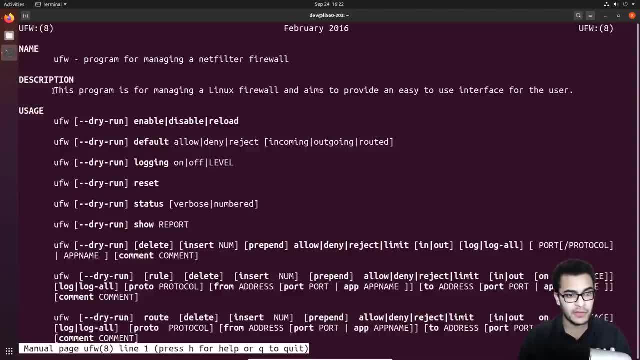 UFW is a program for managing a net filter firewall. This program is used for managing a Linux firewall and aims to provide an easy to use interface for the user. So that's really the. the crescendo of UFW is that, the fact that it gives you a very easy and understandable syntax. 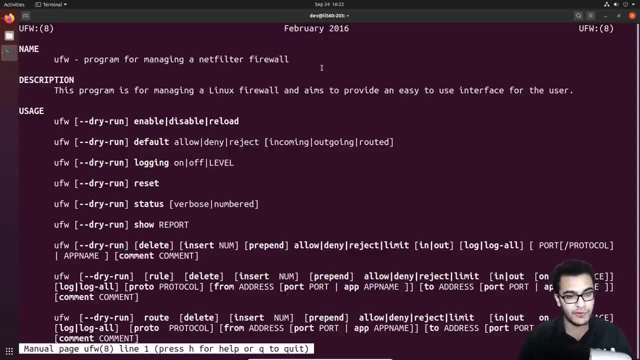 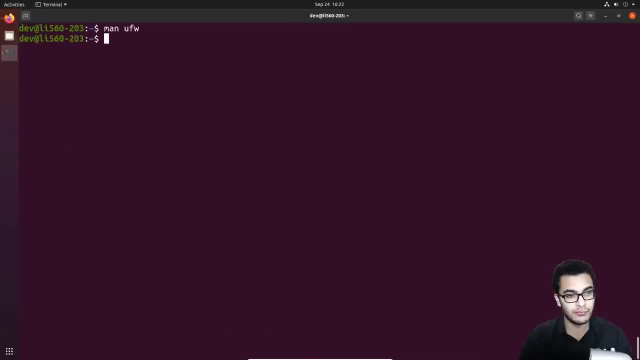 to work with, where, in regards to setting up, you know your various firewall rules. That being said, we can actually go ahead and start taking a look at some of the most important commands. Now, the first thing you want, you need to, you need to take into consideration is: 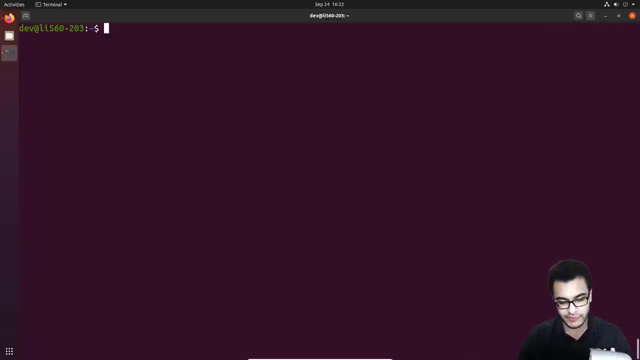 the fact that UFW is a service. Now, when we talk about services, you can start services, you can stop services, you can restart them and you can enable them to actually be actually be run on the system startup, And to do that we, we can use the. 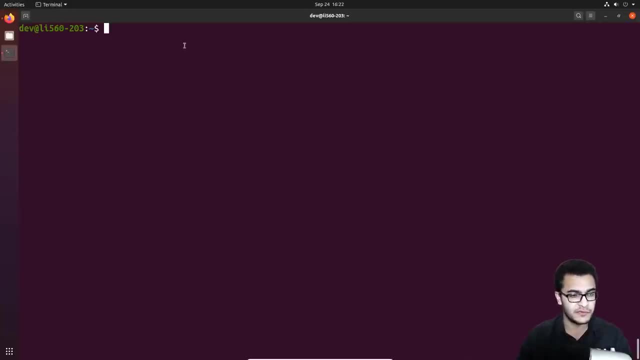 various init systems that come with Linux. In our case, we're using system control, And that's going to be the likely choice for most of you. So the first thing you want to do is, before you be, before you go ahead and start setting up any- any of your rule sets is you need to understand that and you 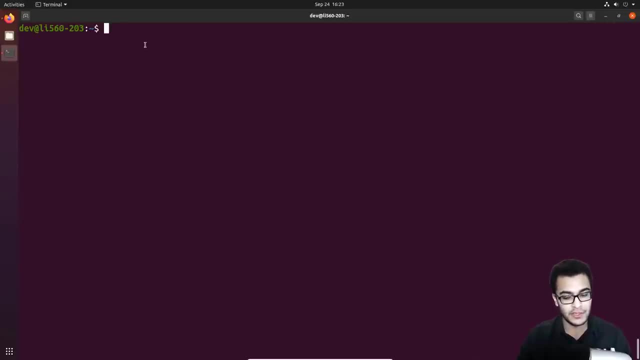 need to make sure that you do not enable the. you do not enable the UFW service before you've set up your firewall rules, because it can actually lock you out. So that's something you want to take into consideration there. That being said, I'm just going to stop talking and we can actually get. 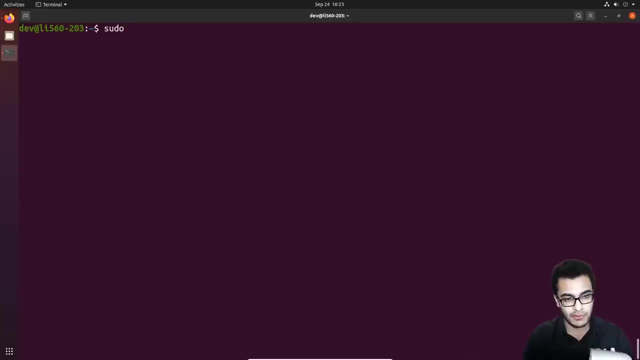 started So we can run the command with. the does require root privileges. So we say sudo UFW And we can take a look at the status. right, So the current status is telling us that it is active By default, I believe, with the. I believe this is the default scenario With this particular Linode. 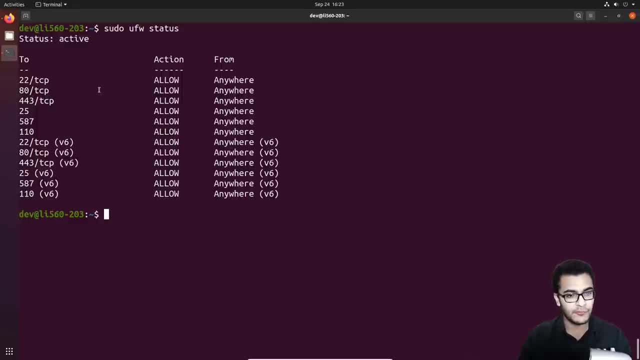 it does come with UFW set up And of course you can see we have both IP v4 rules and IP v6 rules And it's sorted out in the form of the protocol or the port and the action and from or where the 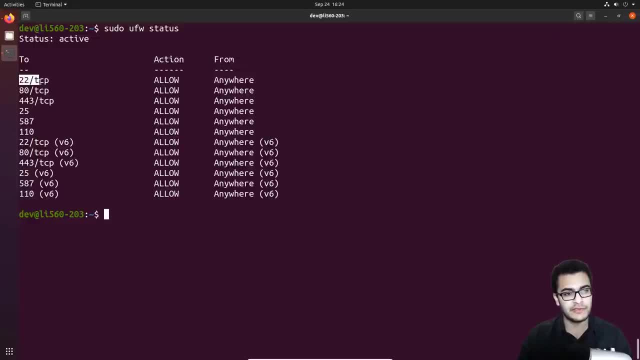 the traffic is coming from. So, for example, we have an SSH port And this of course is TCP And the action is set to allow. so that means SSH is allowed to connect to the server from any IP in the world, and so on and so forth For all the other various ports: port 80,, port 443,, port 25,. 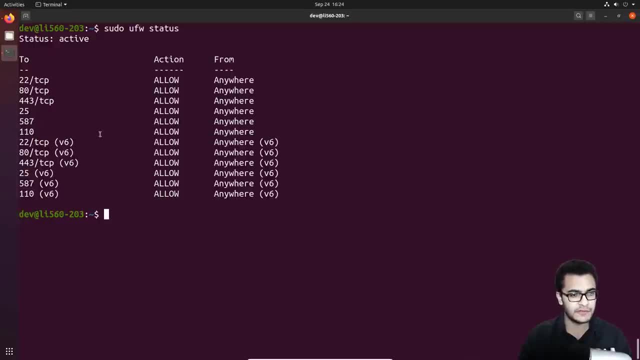 for SMTP, or 5587,, 110, etc. And then, of course, the same is repeated for IP v6.. Now you can modify the default UFW configuration file by going into vim etsy default, and we're looking for. 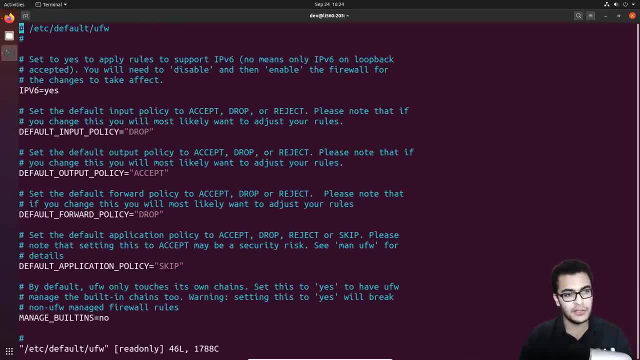 UFW And I'll hit enter And you can enable or disable IP v6.. If you want that, it's recommended to have it running, which, again, we'll leave it as it is. you can also set the default input policy. 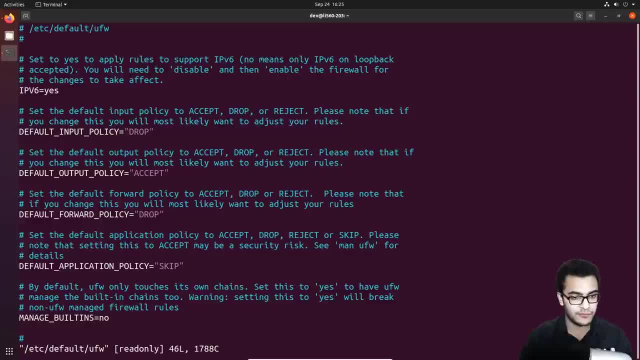 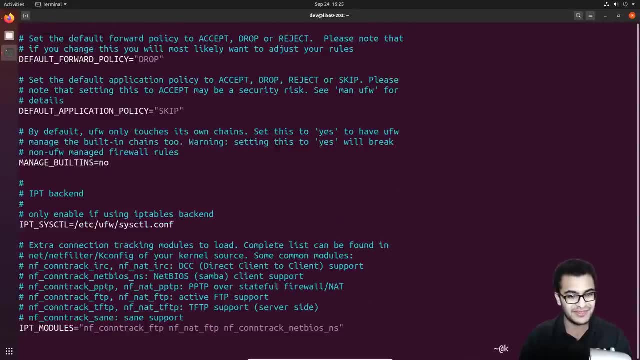 to accept, to drop or reject if you want. And again, you can do that for the default output policy, the forward policy, the application policy, so on and so forth. So the configuration is fairly simple. It's fairly simple to set up. Now what we are going to do is we are going to 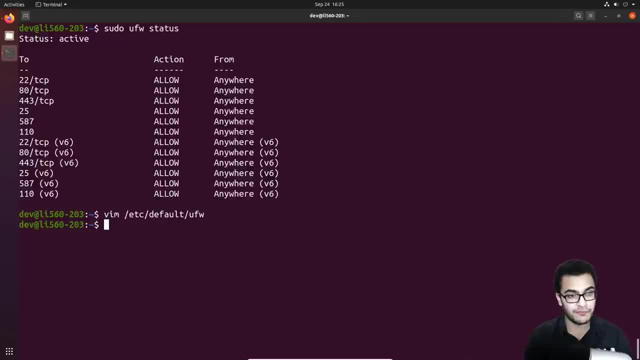 get rid of the current. we're going to get rid of the current configuration. So if we, if we take a look at the status, you can see the current status is active. So if we say sudo, sudo, UFW disable, so we'll disable the service And you can see it's going to tell us the file is stopped and 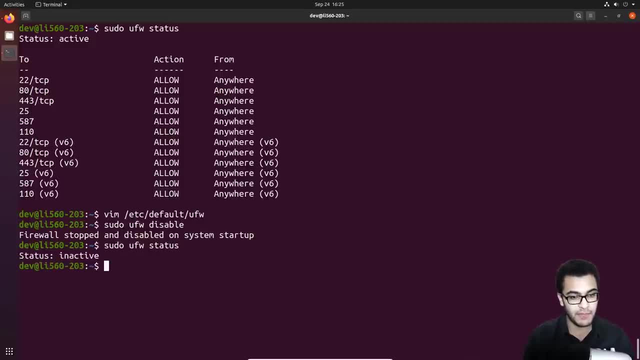 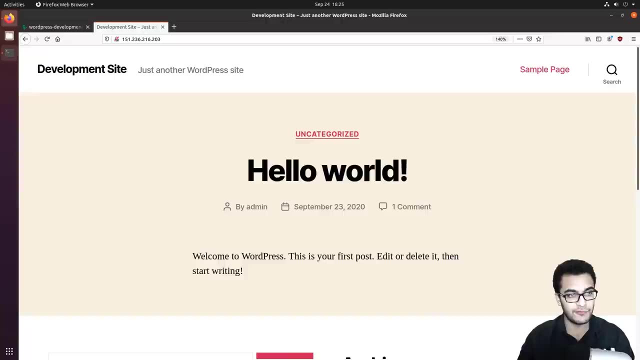 disabled on system startup. If we take a look at the status one more time, it's not going to tell us that it's inactive And that really hasn't affected anything in regards to what we can access before. the rules were all set to give us access anyway, So it's always recommended when setting up. 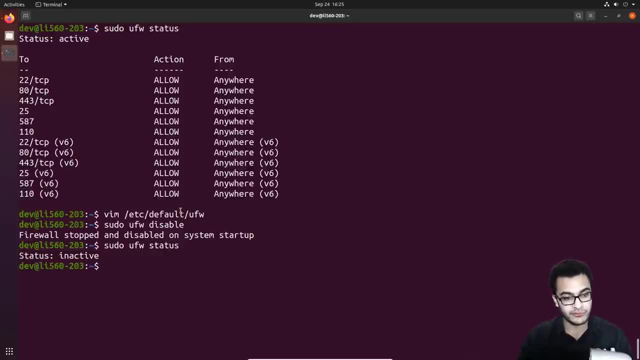 a firewall, especially one on a server, to set up everything from scratch, because it's these type of rules that have been pre configured for you. That can be. that can really cause an issue, because you may forget to disable one or you may have ones that you don't understand that are currently set. 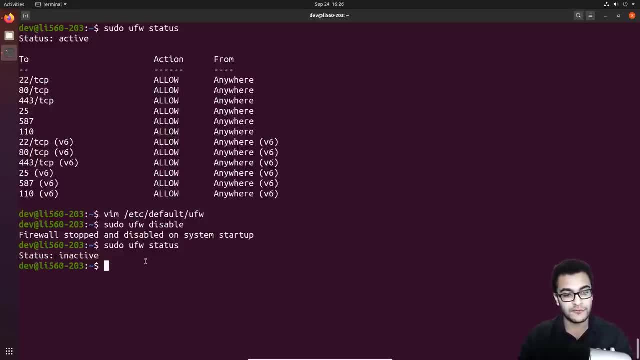 up. So it's always good to start a fresh. And to start a fresh, we need to reset this. So we say sudo, reset right, And that will reset all the, the, the, all the setup rules And it's going to tell. 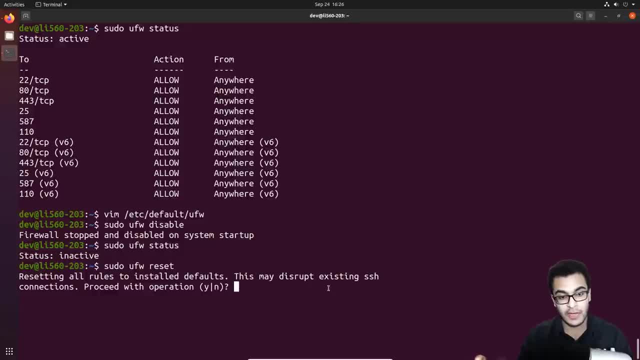 us. this may disrupt existing SSH connections And it's going to ask us if we want to proceed with the cooperation. this is very important. So before you reset the rules, ensure that UFW is disabled so you still have access to the server. So I'm just going to hit Yes And that's going to delete. 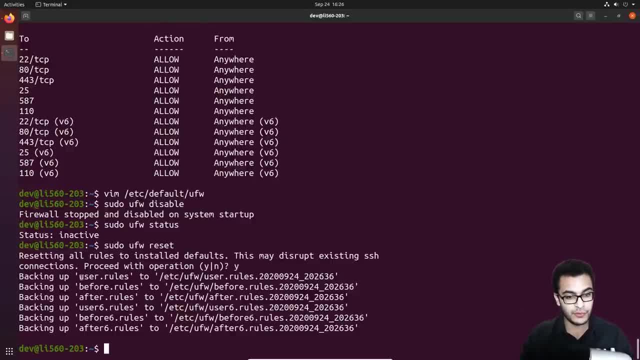 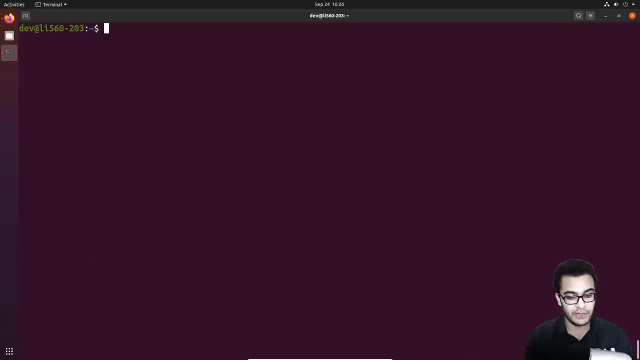 it And you can see it's going to backup the rules into user dot rules And it gives you the directory here. So that's just in case you want to revert back. So again, if we'd say sudo UFW status you. 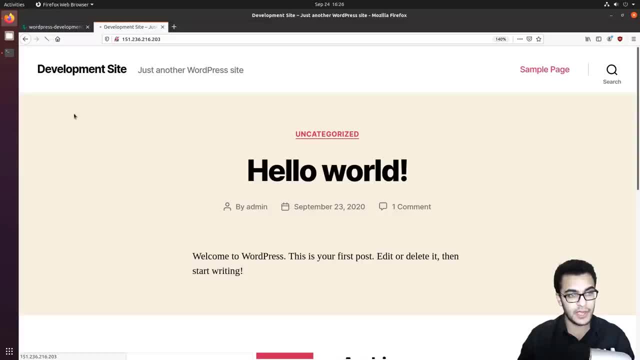 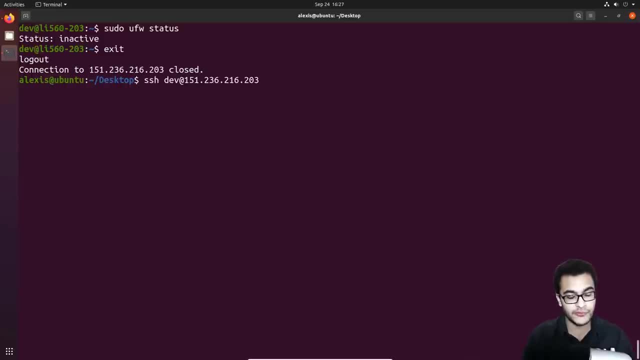 can see it's currently inactive And we can then take a look at the web server. you can see it's still working. If we exit from here and we try and reconnect via SSH, we should be able to still have access, Right. So I'll just set that up And there we are. we still have access and we had 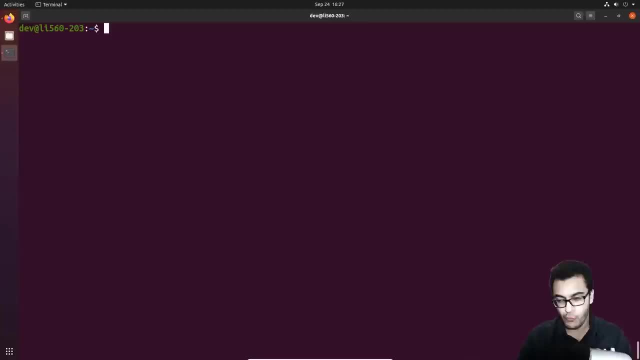 secured it with our SSH key. Now we can actually get started by setting up the default policies, And this is recommended for every fresh configuration. So the default policies are as follows: the default policy for incoming connections is that we deny them, And the default policy for outgoing connections is that we allow. 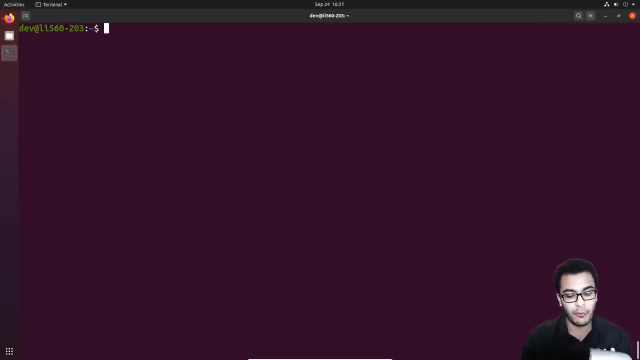 them. So we'll set that up And then after that we'll start configuring our own rules. So we say sudo UFW And we say default, deny out incoming. So sudo UFW, default, deny incoming. And don't worry, if that doesn't make sense, we'll, we'll be. 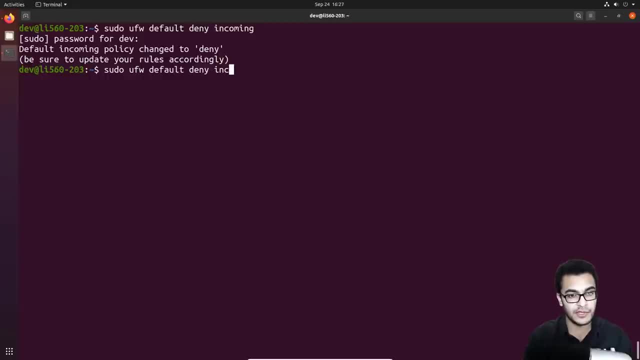 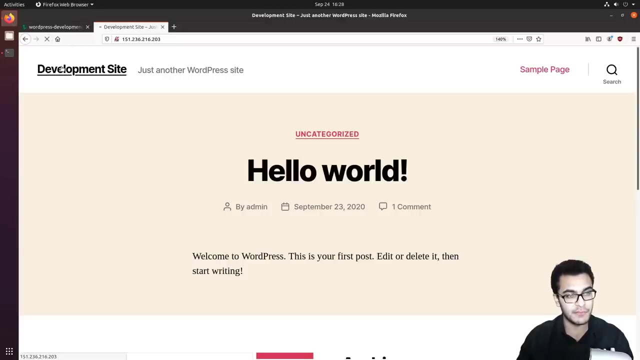 changing all of this And we can then say: sudo default, allow outgoing right. So we say allow outgoing And remember this is still. what's happening is the UFW is currently disabled, So it's not going to affect anything as of yet. So if I try and restart the server, you can see we should. 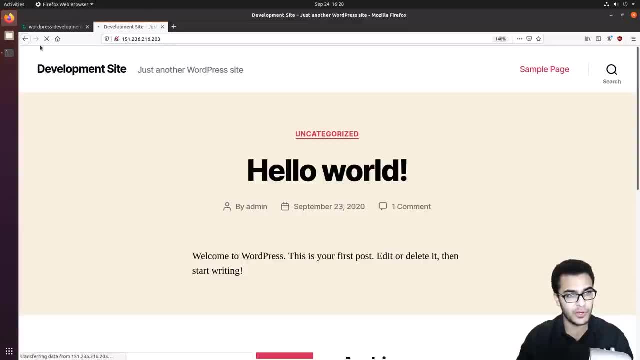 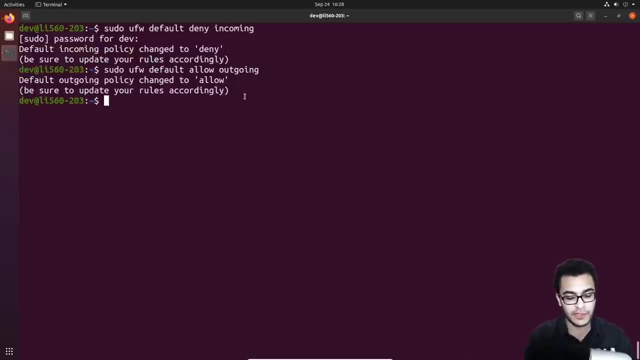 still have. we should still have access if it's. if it does not work- And we can see that that's still working. If it doesn't work, what we can do is we can disable the service completely. So we can say: sudo system control status. UFW is going to tell us that it's. 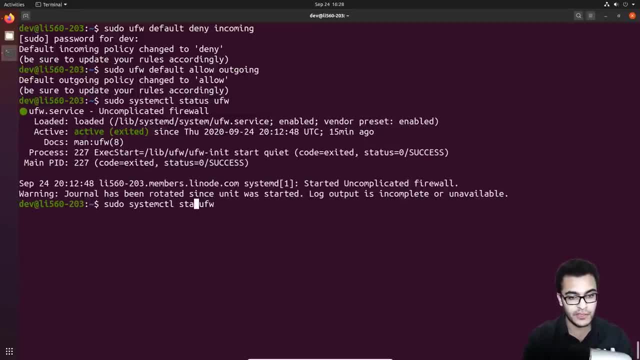 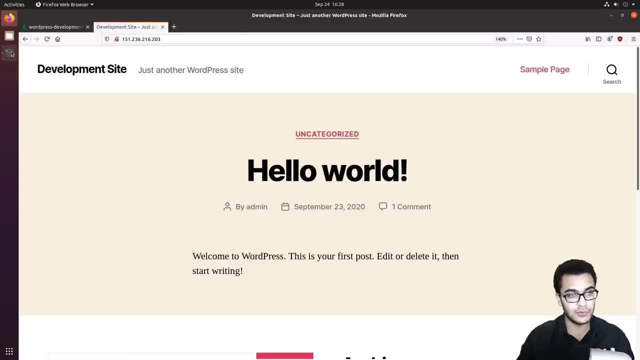 loaded and active, So we can disable it in the meantime, So we can say stop, Right, and we're going to have that stop And again, that doesn't affect anything yet. So it's very important that you, you actually disable everything, you set your rules and then activate it and see if anything is. 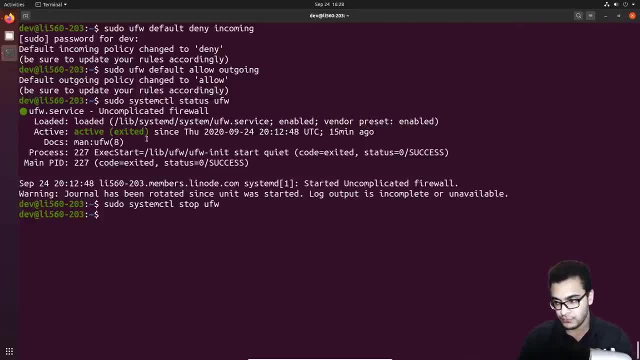 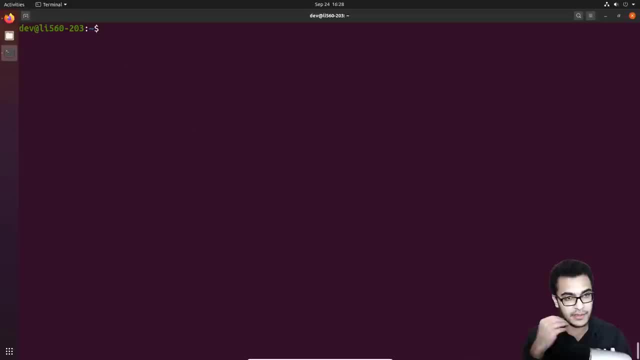 causing any issues. So that's the first step here And we've set up the default policies. The next thing we can take a look at is if we take a look and we see we say sudo UFW status, we can display that it's going to tell us it's inactive. So we can. 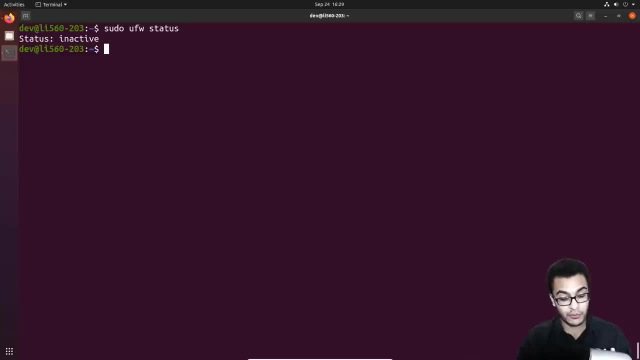 start adding our rules. So, when adding your rules, when configuring your various rules for your firewall, it's very important that you understand what rules or what services you want to keep active in regards to incoming and outgoing connections, and what and what services. 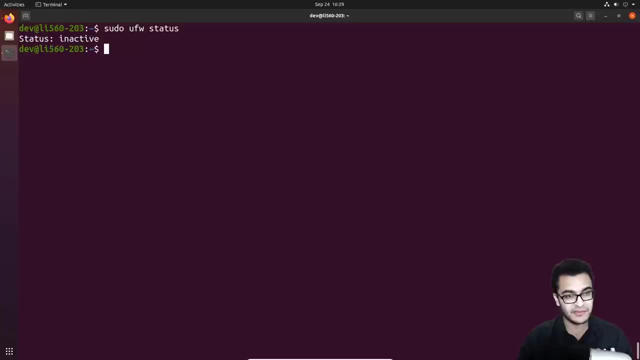 and protocols you want to actually disable or prevent from being accessed. In our case, we know that the two essential protocols that we want to keep active are going to be HTTP, both on a port 80 and port 4434, HTTPS and port 22 for SSH. So to do that, we're going to say sudo. 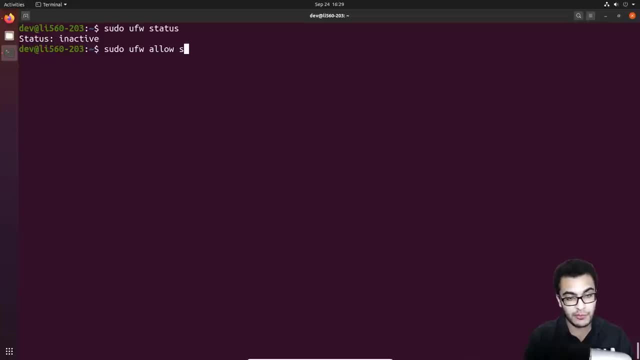 UFW allow And we can specify the protocol either by saying SSH or by the port number. In this case we can simply just say SSH, hit enter is going to say rules updated for both IPv4 and IPv6.. We can then say UFW status And again it's going to tell us it's inactive And 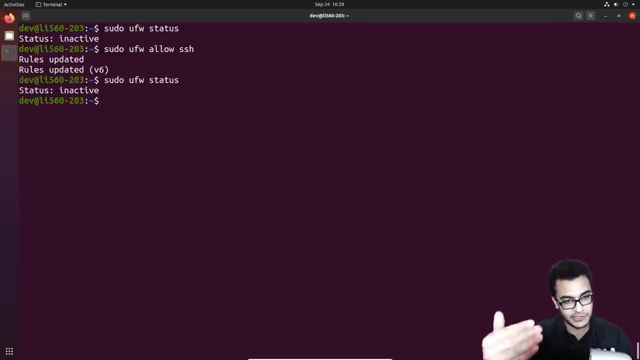 once we enable it or we start it, we will actually list out with the various rules that we have. The next rule we want to allow is going to be HTTP, So that's both port 80 and HTTPS, even though we haven't configured an SSL, SSL certificate yet. So these are the most important. 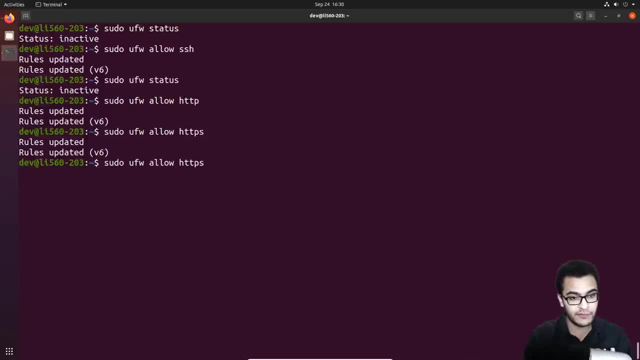 rules And of course we can allow any other ports that we want. So for example, if I wanted to allow FTP, I can say FTP like so and we don't have FTP running on the on the server. But again we can do. 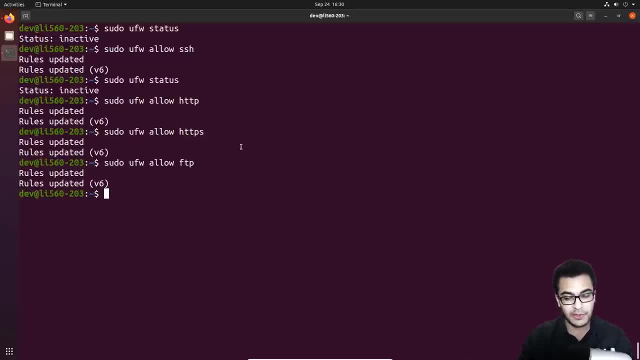 that as well. If we want to allow a particular connection from an IP address- like, let's say, we only want to allow or we want to allow a connection from a particular IP address explicitly- we can define that so we can say: sudo UFW, allow- sorry, let me just correct the syntax here. So sudo UFW. 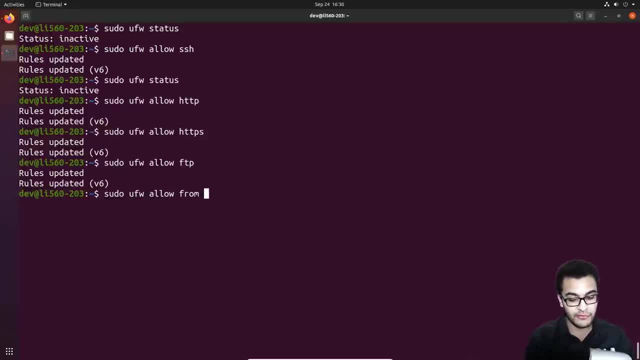 allow And then we say from and we list out the IP address right over here So I can save 10.0 point 0.1., For example. I can do that right over here and it enter: it's going to say rules updated. 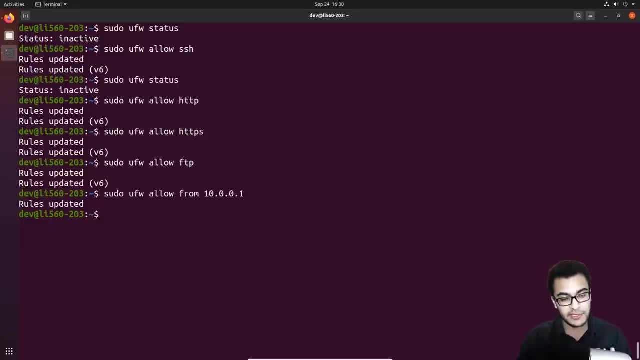 I can also specify to. I can also explicitly define a rule that allows a particular connection to a particular port. So let's say I deny all SSH connections but I only allow an SSH connection to connect And I can modify the access port amount. So today I'm going to need a data under 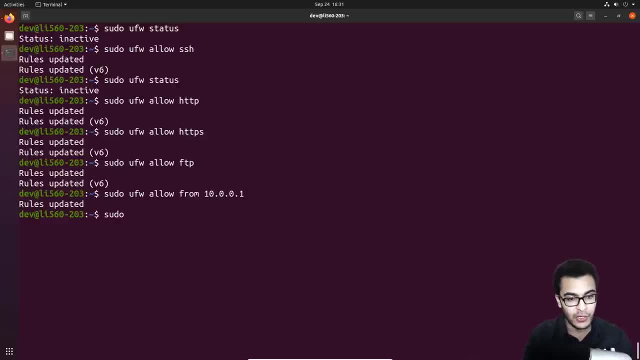 IP address. So I do not allow that and just leave that as path. So something like that. I can make it compared either, So I can go ahead. I can choose an IP address name, taste it, then go ahead and take that name change simple. So are tablespoon friends even so. 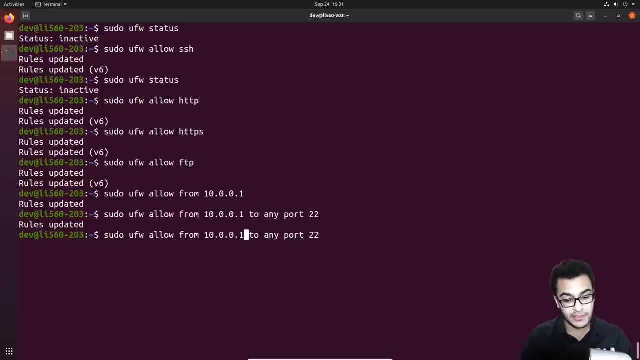 it will be a different kind of thing, but if you click on it and I hit save, now we can see all our phone lines have some different pickups, And then we see that we have the IP class, the 24.1 line. 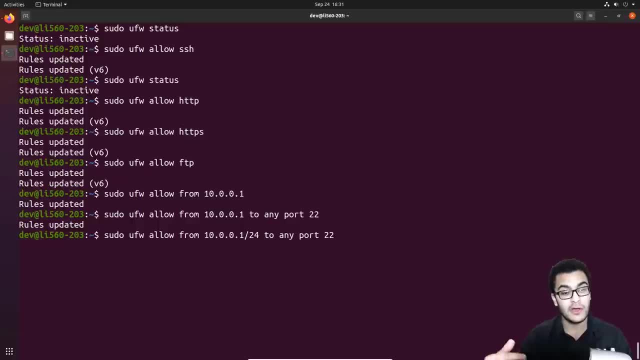 that you'll be using or that you're setting within your rules. These IPs have to be static and not dynamic, because if you set up your firewall to allow connections from your IP address and your IP address changes, then you'll not get access because the rule has been set for that IP alone. 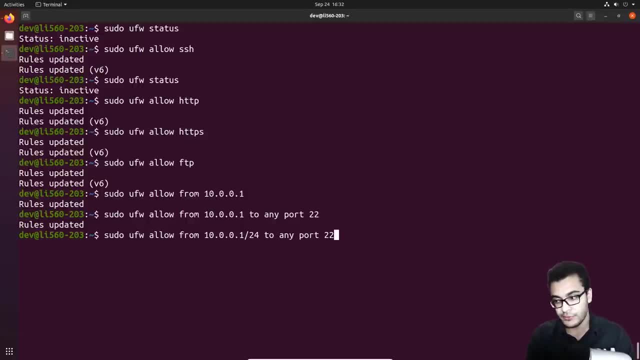 So you can also set subnets if you want. I'm not going to do that right now, I'm just simply showing you how to do this. So that's essentially all your rules: to say that that will allow these particular services that were stated explicitly. Now, after we've done this, we don't want to deny 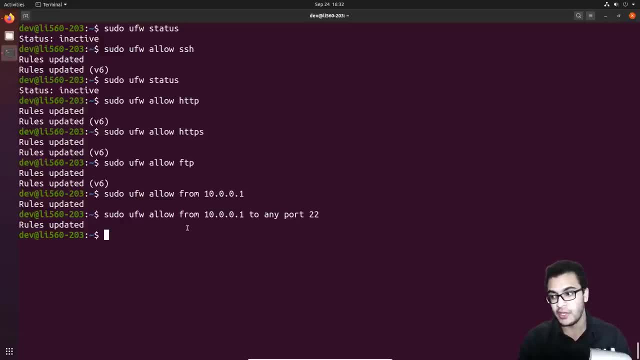 anything yet because by default all incoming connections have been set to deny. That was the default policy configuration that we set up earlier. So what we can do is we can say sudo system control, start, and we say ufw, And we can then say sudo, ufw, enable, ufw, enable. 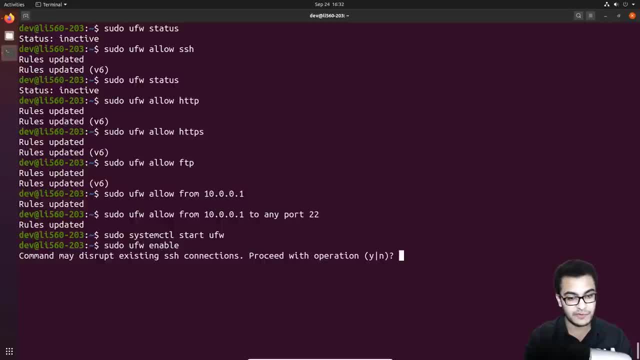 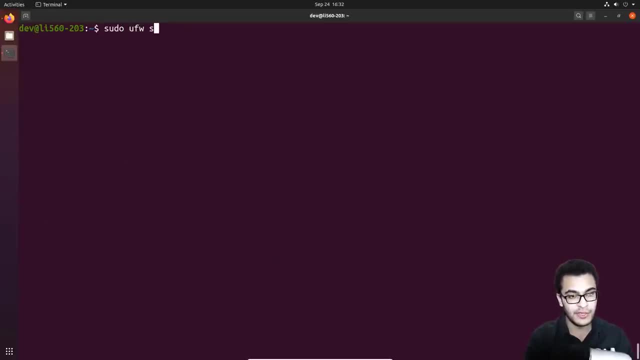 Like so And it's going to say these: this may disrupt existing SSH connections. I'm going to say yes, And the firewall is active and enabled. If we now say sudo ufw status and we hit enter, it will now going to list our the various rules that we have configured. So you can see that for. 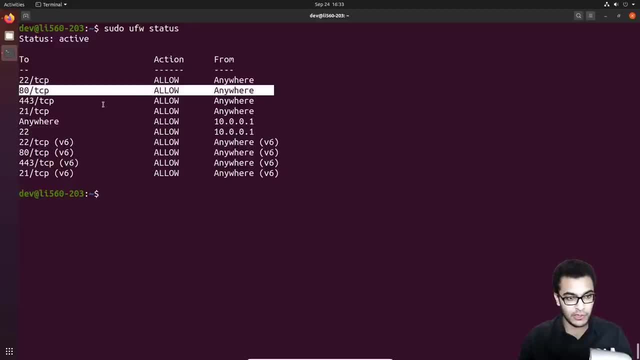 port 22, that is set to allow port 80 set to allow. port 443 allow, port 21 allow. and then we are allowing any connection from this IP right over here, which is kind of a useless rule. I was just adding it there So you can understand what's going on. And then, of course, we can. we. 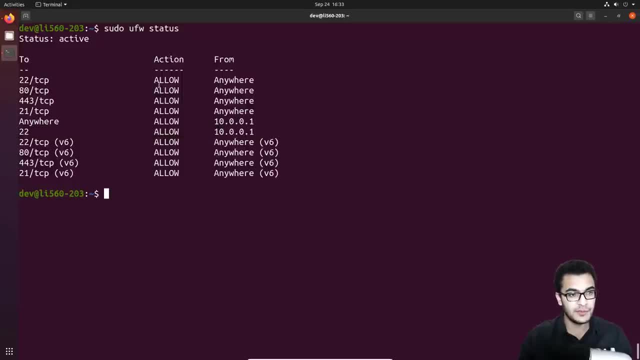 allow all connections to port 22 from this particular IP. So if we try and access our web server now, we should have access to it immediately, like so. And again, the reason I'm doing this is just to show you that it is working. So if I try and connect via SSH here you can see. 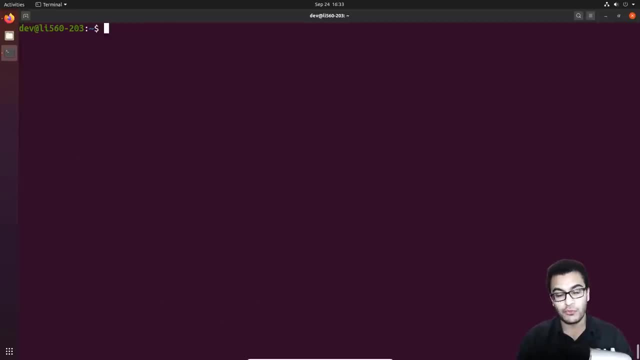 that works as well. So those are, that is, how to allow, or how to set rules to allow connections If we want to. if we want to start denying connections to services, we can say, for example, let me just say: sudo ufw. And if we want, 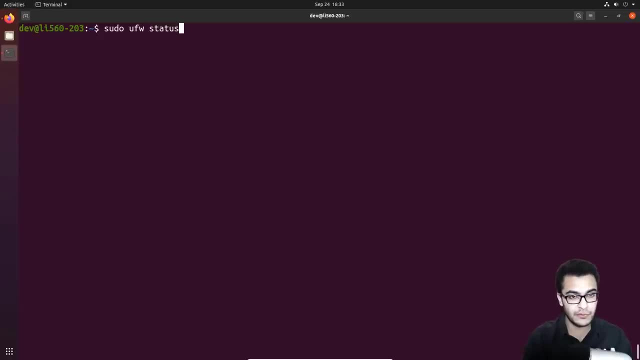 to list out the rules and delete certain rules. we can say ufw- status numbered. we can list out the various, the numbering for all of these rules And then we can say sudo ufw- delete and then specify a rule number. So in our case, what we can do now is we can start getting rid of rule five and rule. 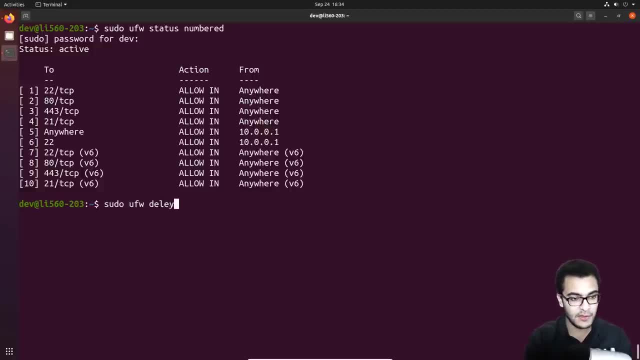 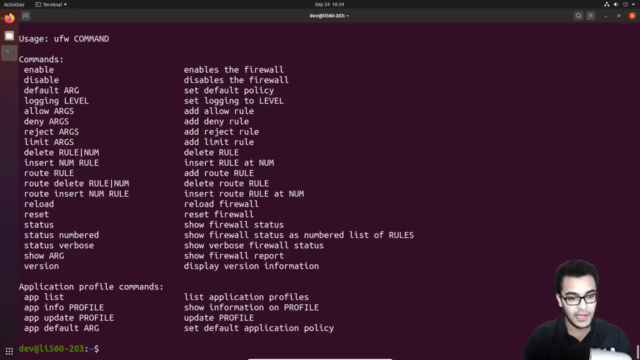 six. So sudo ufw. and we say delete, sorry, delete rule five, right. So delete rule five because we don't need that And it looks like we have an issue. is sudo ufw, delete? And we just specify the option. 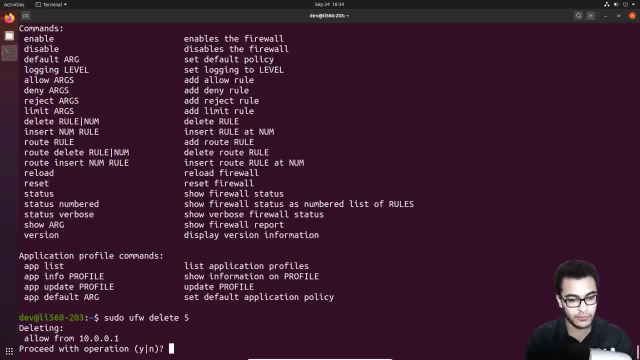 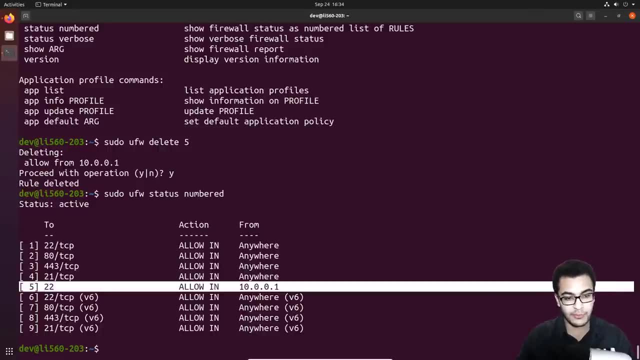 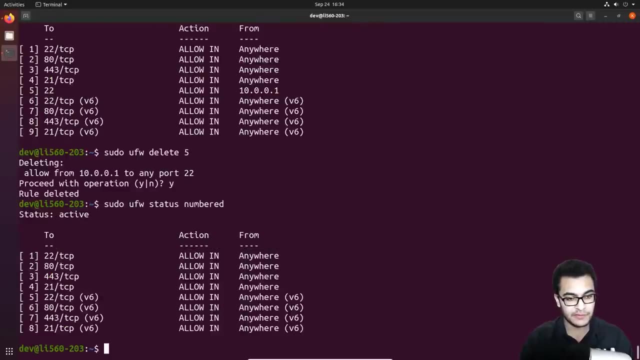 five here And it's going to say deleting: Yes, we want to do that. And we then take a look at the status again. we then want to disable rule five again because it's moved upwards one more time. So we hit enter, that's going to delete that. And now, if we take a look at the status again, you can see the. 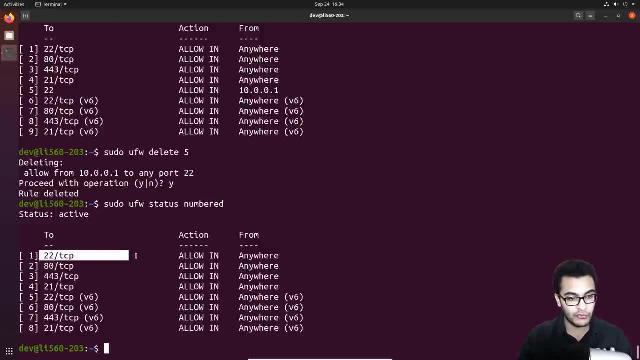 only the only rules that we have are going to be port 22. So that is allowing SSH connections. we then have port 80,, which allows HTTP connections, port 443,, port 21,, which is FTP, So we can also get. 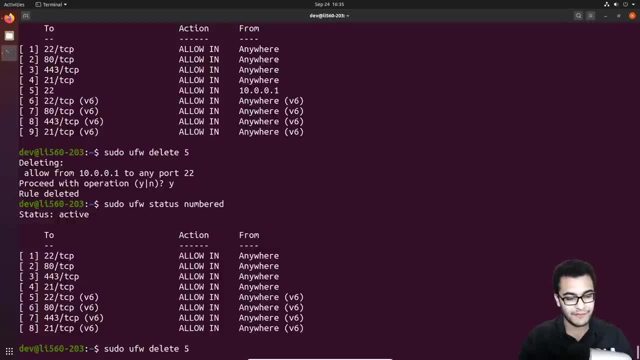 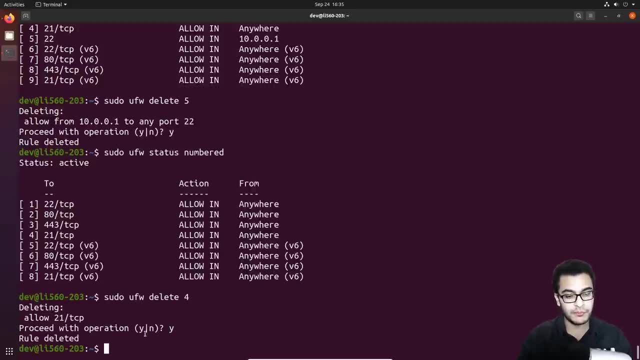 rid of port 21. Because we do not have. we do not have FTP running, So we can delete that. And now it's becoming much more clearer. So, just for an example, if I want to deny all connections to the web server, I can do that very simply by first of all listing out and I can say: I wanted to. 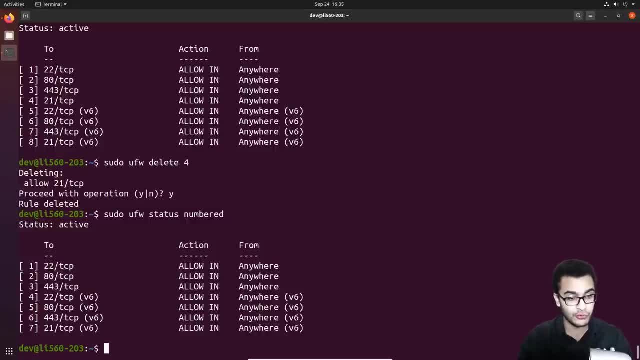 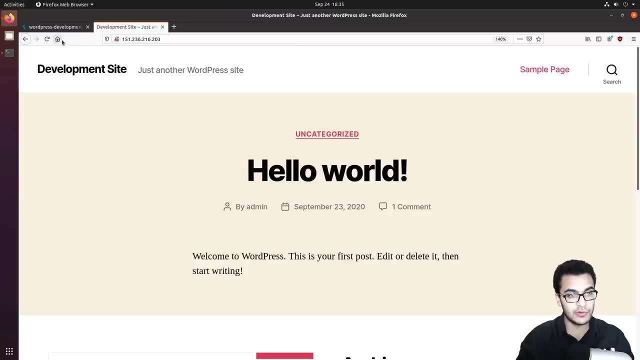 I want to delete the rule 22, or sorry, the rule to not 22.. So I can delete that. and that's port 80 for HTTP, And if I try and reload the web server now, we'll just wait for that to reload here. 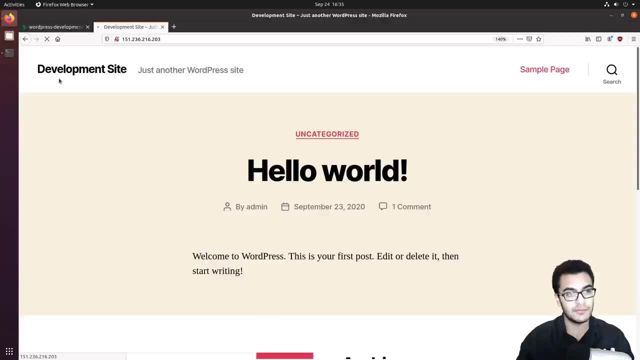 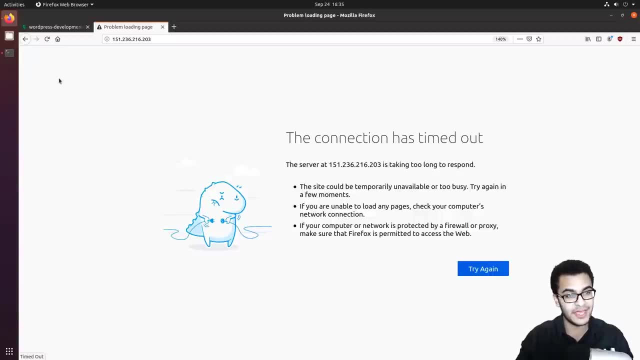 And you can see I have no connection Coming back. So that means I've- I've again, within the firewall, I've configured no access or no incoming access for the port 80. And you might be wondering: well, we haven't. 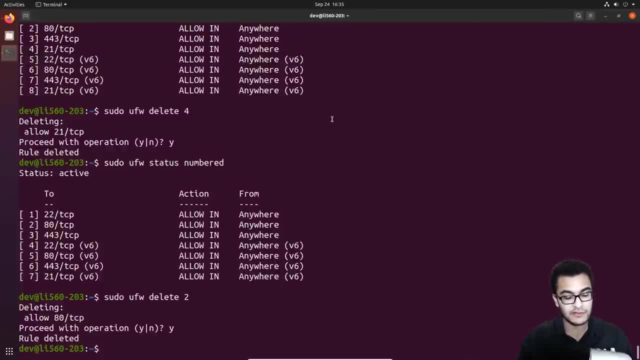 actually configured that manually. The reason that is is the case is because when we were configuring the default policy lists by default, if you remember, what happened is we configured all incoming connections or we configured the firewall to deny all incoming connections unless we explicitly define otherwise or we explicitly allow it manually. In our case, we allowed only 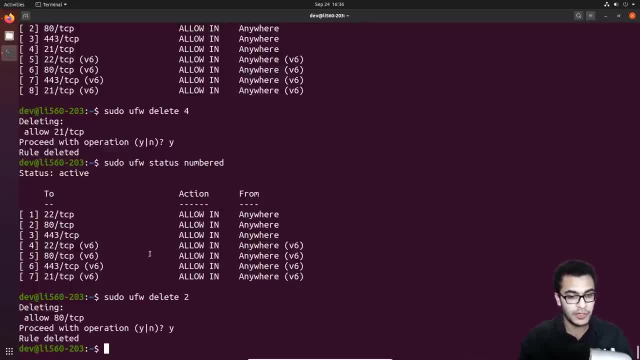 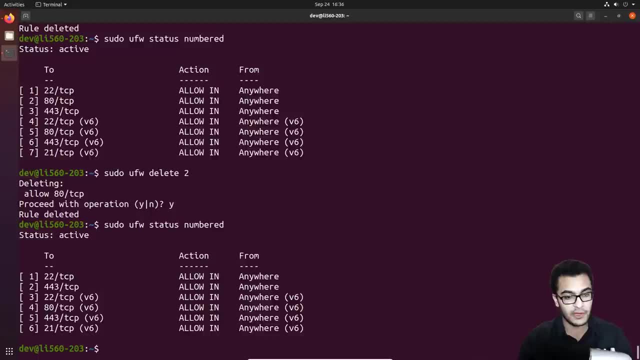 port 22, port 80, port 443, manually. So those are the only ones that are going to be working. So, again, if I list out the status one more time, if I now enable it, so I say sudo, ufw, enable. 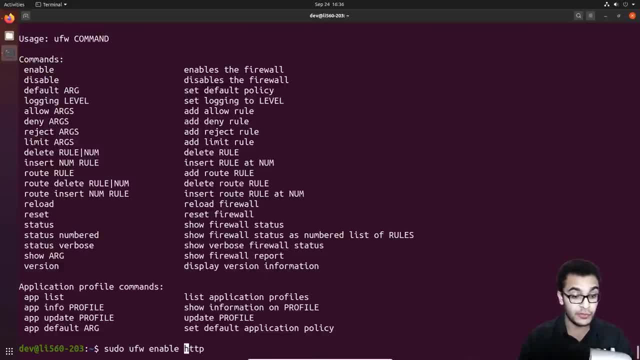 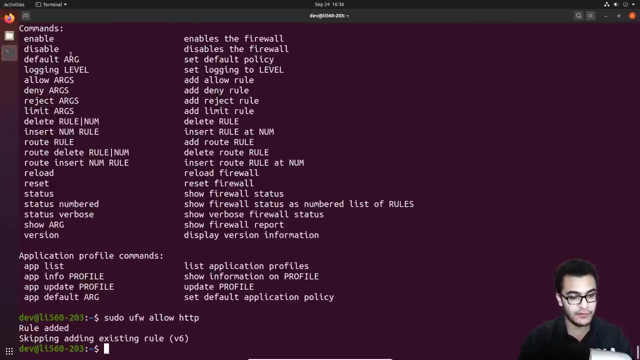 HTTP and hit enter. Sorry, sudo not enable. we want to allow it, my bad. the syntax is much more simpler, So allow and it's going to add the rule. And if we now try and refresh the web server, you can see. 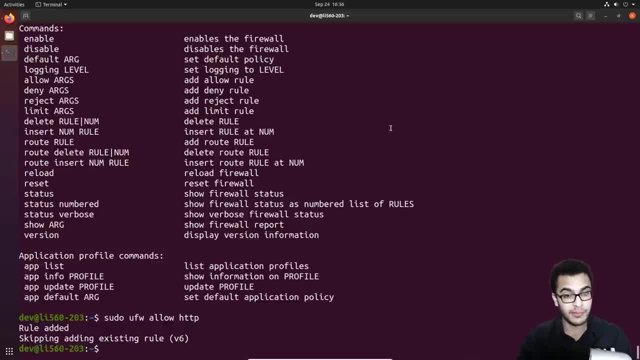 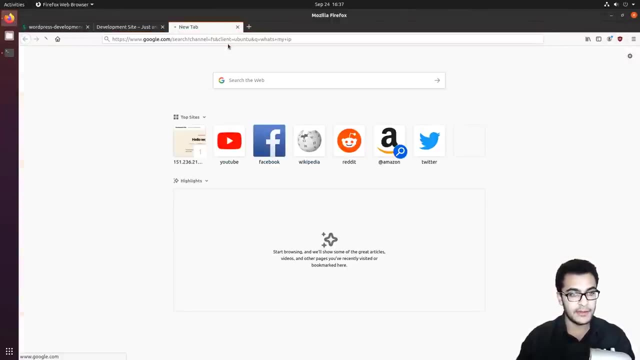 it now works. Now we can also allow, as I said, from a particular IP. So if I will only want to allow my IP address access to that particular, to the web server, what I can do is I can get my, my public IP address- So what's my IP? And I can just, you know, copy that And, of course, 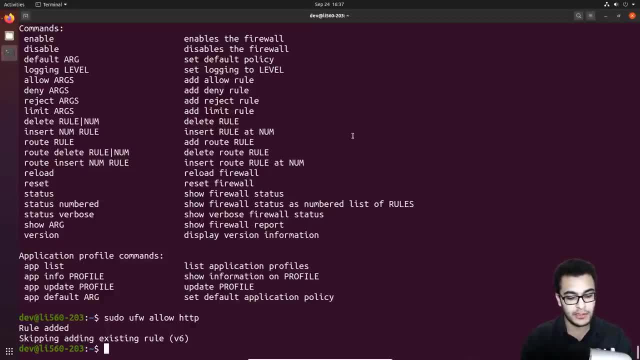 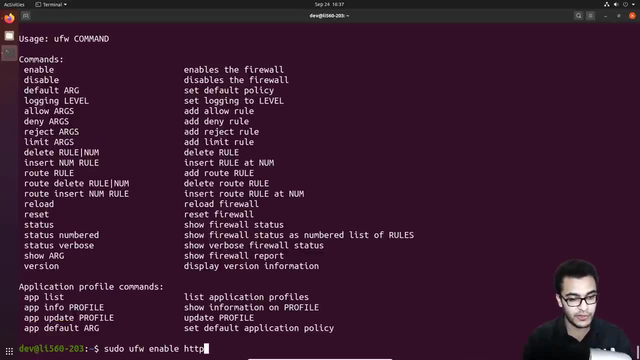 I can then just go back into my terminal here And if I say, if I list out the rules, because I want to delete the rule that allows all connections, So for example, if I go into the status here and I want to delete this rule number three, 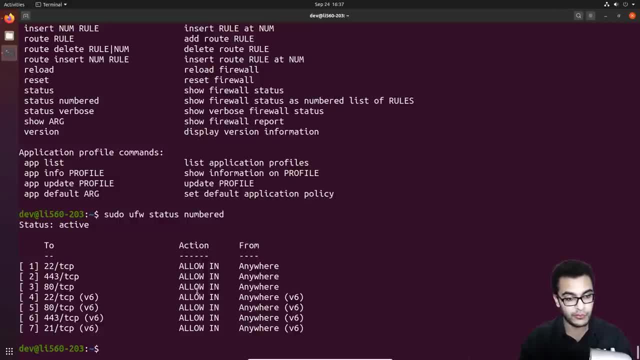 because that's allowing any connection to the port 80. So we want to get rid of that and then explicitly define that only my IP has access to that port. So I'll say sudo, ufw, delete or 80, right, so we can get rid of that. Sorry, not port 80.. 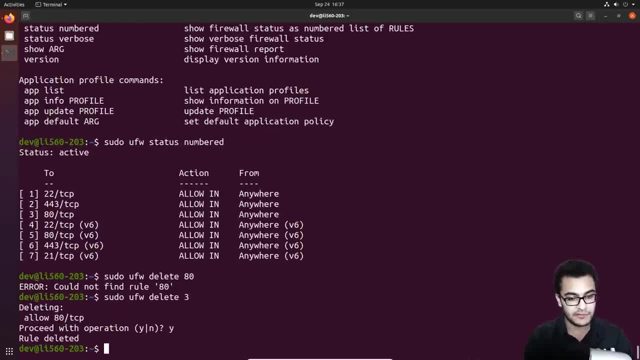 Option number three, And we're going to do yes. And then we want to say: we can then say sudo ufw, allow from IP. So sudo ufw, allow from IP, and we can then paste the IP in here, right So? 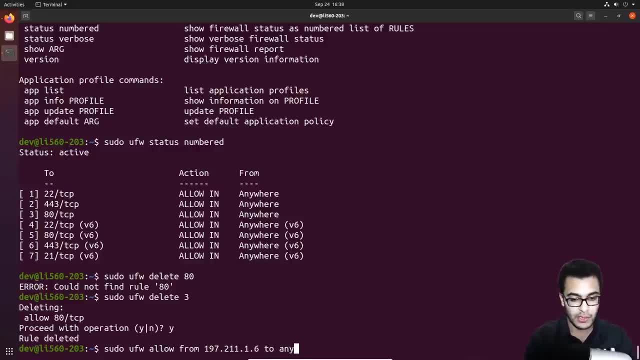 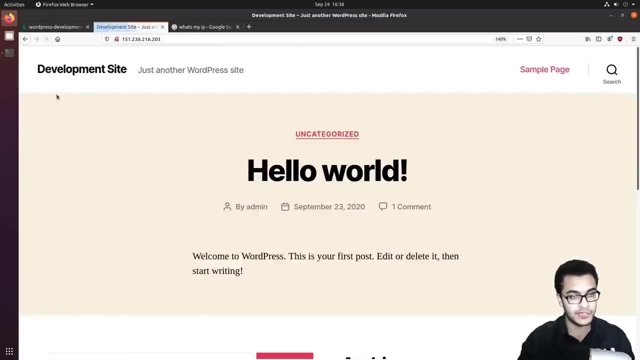 allow from to any port, any port 80, right, and we hit enter and that's going to add it, So you can see now it's going to work. If I refresh this, I'll still have access, And that's because. 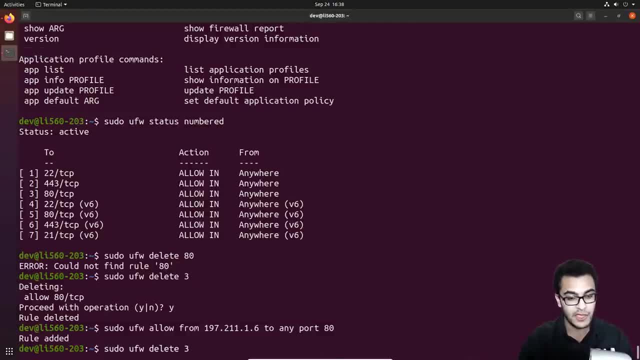 I'm trying to access it with my ID, So I'm going to refresh this. I'll still have access and that's because I'm trying to access it with my ID, With my IP address, if I delete that rule. so I'll just list the status numbered. 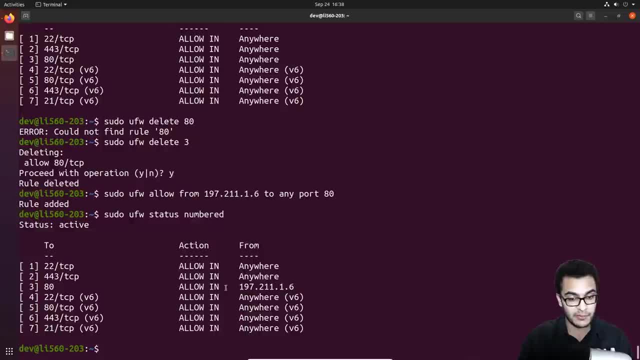 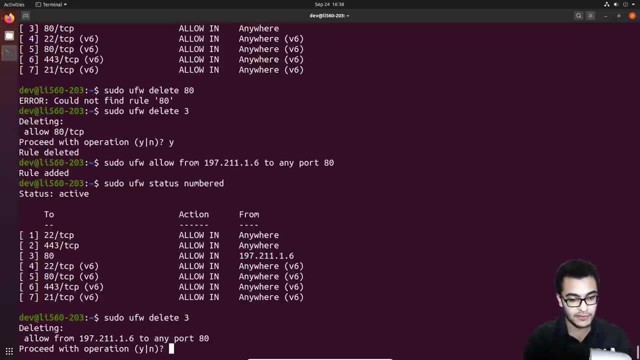 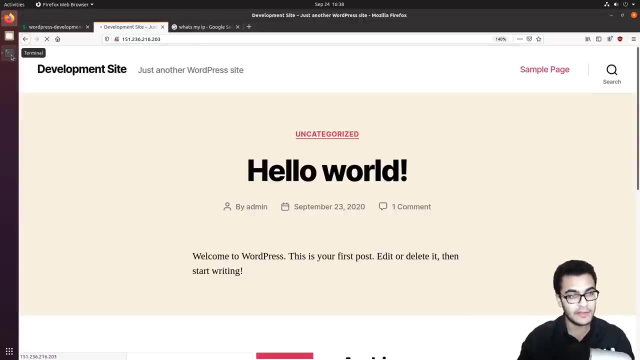 and I delete this rule right over here. you can see it allows only my IP. So I'll just say sudo, ufw, delete, and that is rule three, and I enter that we are, and I try and refresh this. you should now see that we have no access to the web server And I can then re enable the. 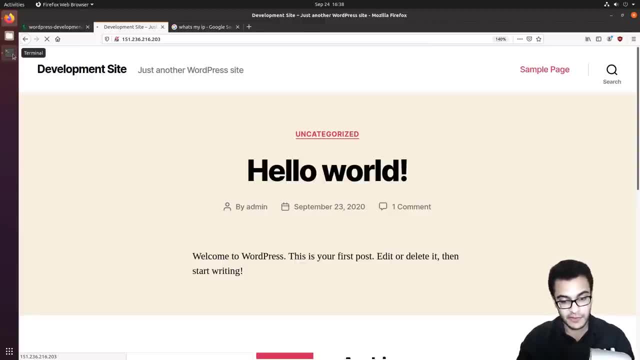 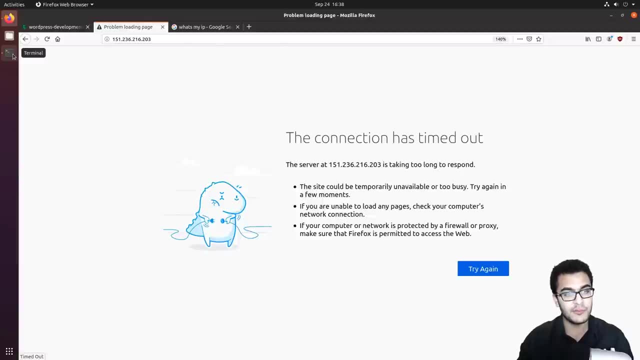 rule that allows any IP address to access it. So this is a great way for IP or administrators of the on the web server to actually disable access to the particular website and only they can access it because they have their own IP. And, as I said, a note of caution. 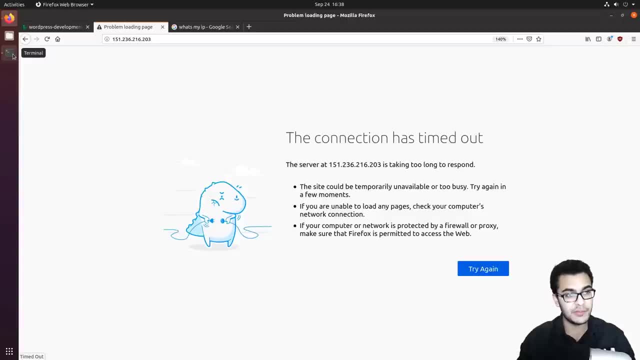 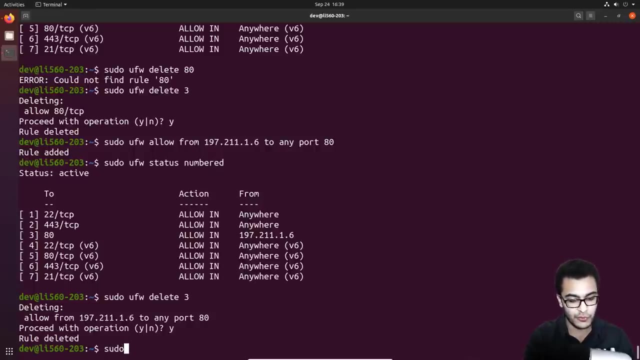 is ensure that you have a static IP. Otherwise, if your IP address changes or you go to a different location with a different IP address, you'll not be able to access it. So you want to keep that in mind. I generally don't recommend running these rules. So again, we just say sudo ufw. 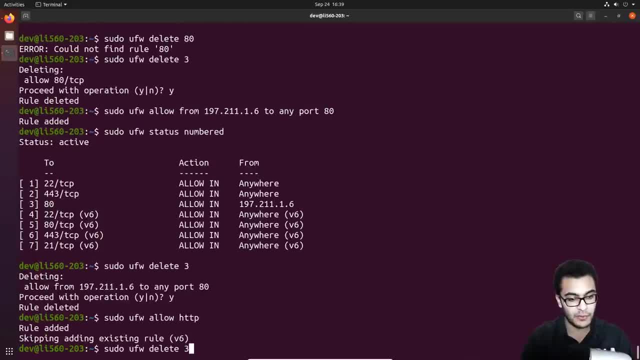 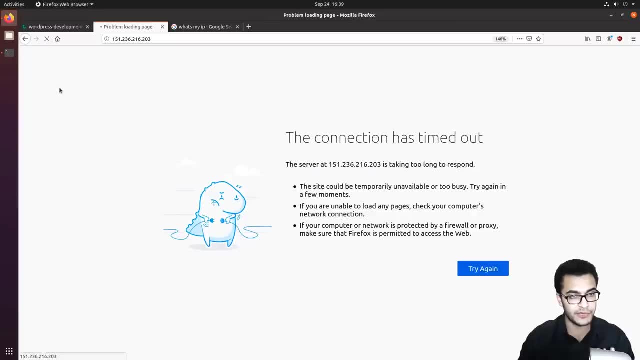 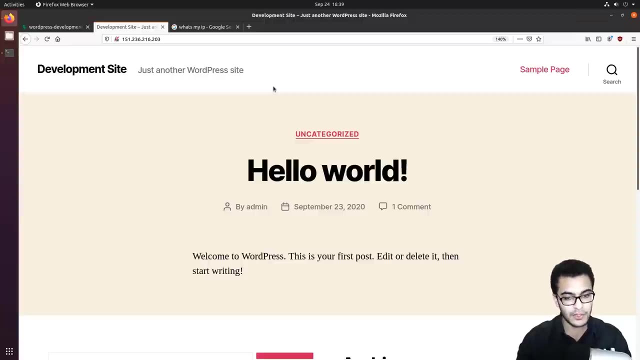 allow HTTP, hit enter, and that's just going to allow anyone to access it. So if we list these, the numbered rules, that's pretty much fine for me right now. So if I refresh that, we still have access. So again you can see how easy it is and how important it is to do to configure rules. 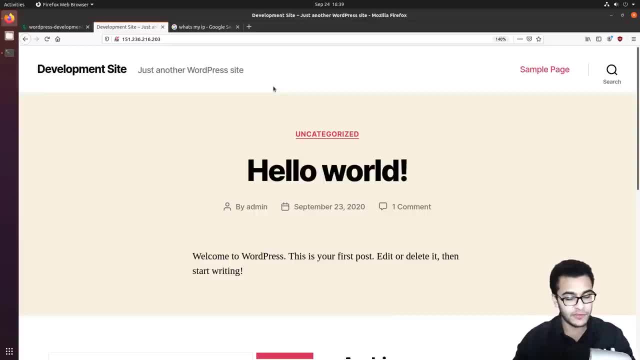 yourself and to understand what's going on. Now. as I said, on this particular web server, the only services we need running are going to be SSH and port and and the web server, And we've we've talked about secure During SSH. we've talked about securing the web server. we can also limit SSH access to our IP. 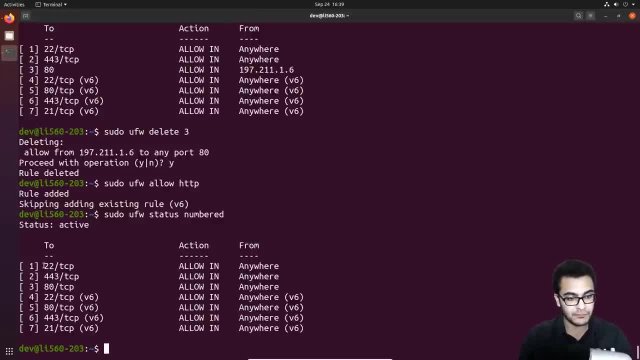 And to do that all I would need to do is just delete the the SSH rule here and then specify. I can just say: sudo, ufw, allow from my IP address to the port 22. And that will only allow my IP address to connect via SSH. So that's fairly simple And, of course, 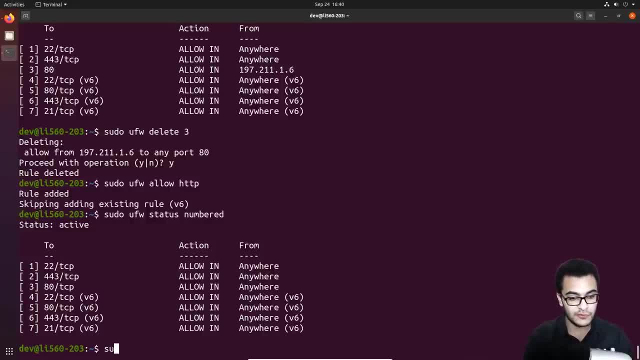 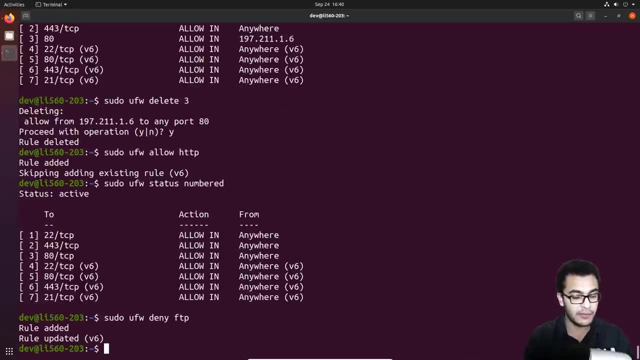 I can deny any particular service. So I can say here: sudo ufw deny instead of allow, So sudo ufw deny FTP. So I can deny all FTP connections, all FTP incoming connections, if I want. I can also say another service like HTTP, if I say sudo ufw deny HTTP. 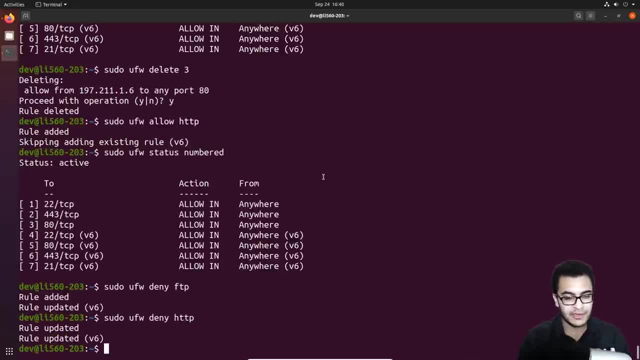 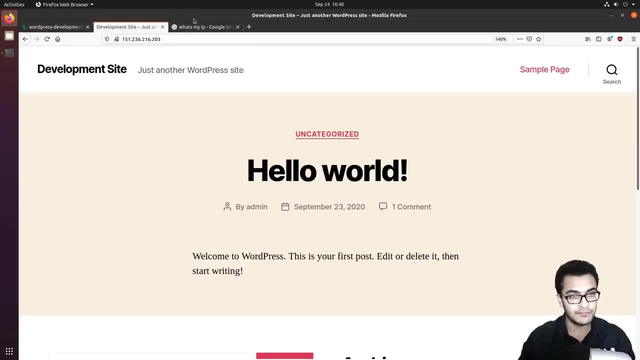 and I enter. I can do that as well. So allowing and denying is very, very simple. If I want to deny from a particular IP, I can also do that. sudo ufw, deny from, and I specify the IP. so deny from. I put in my IP right over here And I can then say to any particular service, or just deny all. 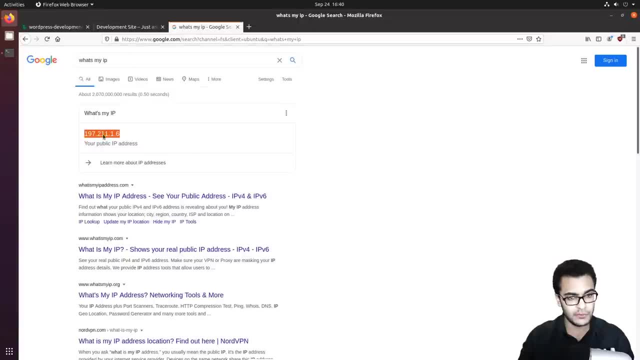 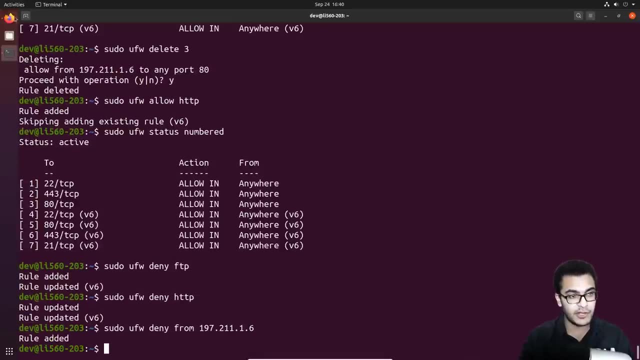 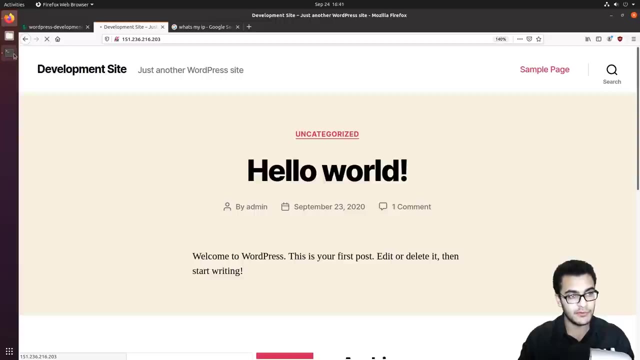 connections from this particular target. So I can do that right here. So you sudo ufw, deny from and then paste in my IP And if I try and access the web server should let me just restart that. There we are. looks like we cannot connect If I go back and I try and exit out of SSH here and I try and 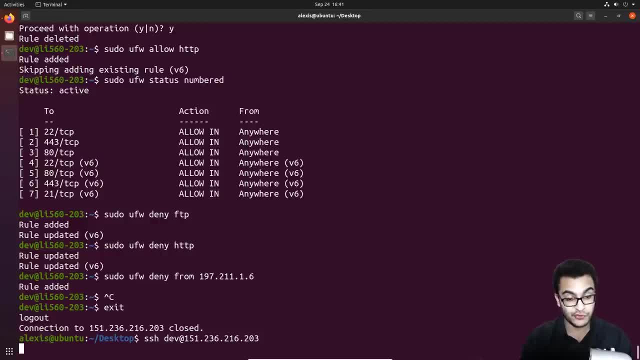 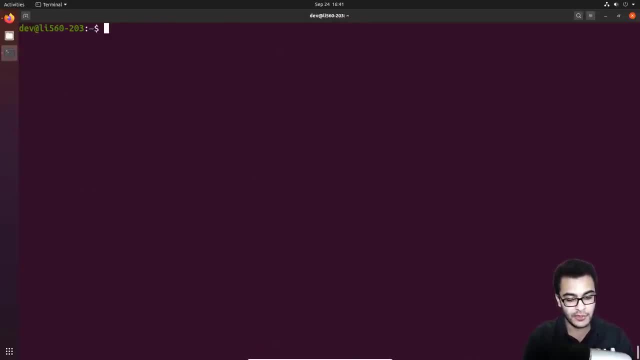 SSH connection. you can see I don't have access. So I fundamentally or essentially, just locked myself with. I actually got access back And that's because if I say sudo, ufw status numbered, there we are, just paste in my password. you can see that it's going to allow any SSH. 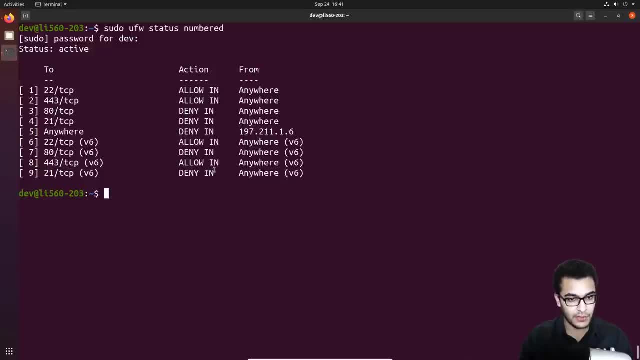 connection. And if we delete that, you can see, once I delete that particular rule it's going to deny all connections and I can then explicitly state a port that I want. So that's essentially how to deny connections. If we want to delete rules, as I said, we can say: sudo ufw, delete, we can get rid of. 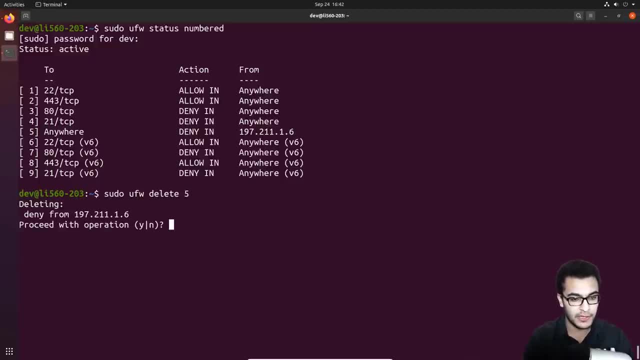 let's see rule number five, because we don't need that. hit yes And we need rule four. we can actually just get rid of rule four because I don't think we need that. that is denied port 21.. ftps. And then we can get rid of rule rule three. so we just get rid of rule three. 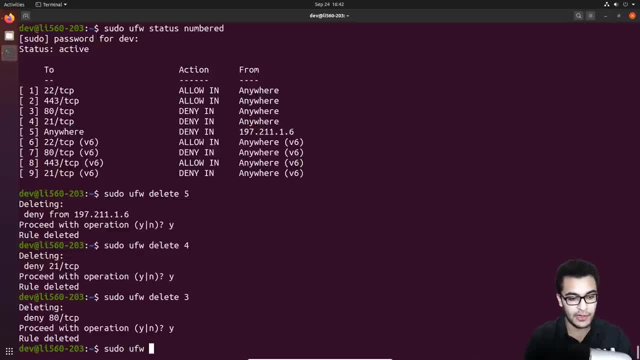 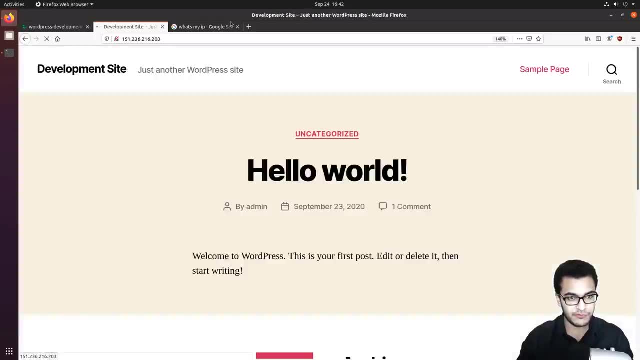 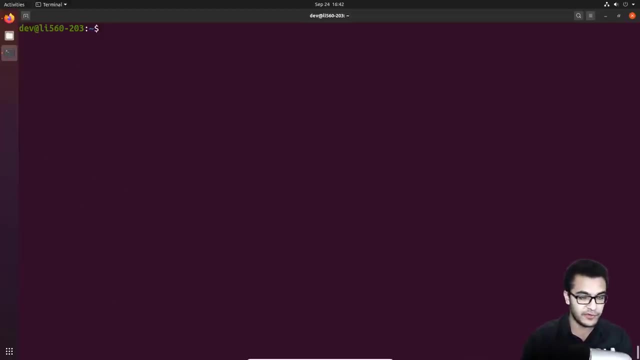 And we can then just say sudo ufw allow HTTP and hit enter. that's going to allow our web server. So we now have access to the web server that we are, and we also have access via SSH. So the key thing to take into consideration here- allowing and denying rules- is very simple. 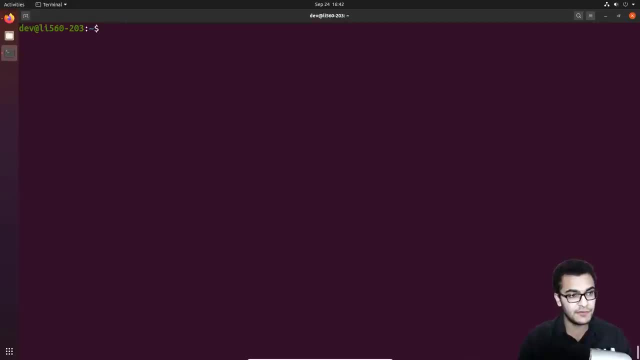 Just know what services and ports you want to keep active, The ones you want to allow connections to and the ones you want to you actually want to protect from active connections. you can specify the IP addresses you want to block. you can specify the IP addresses you want to allow in, But with that you want to make sure that 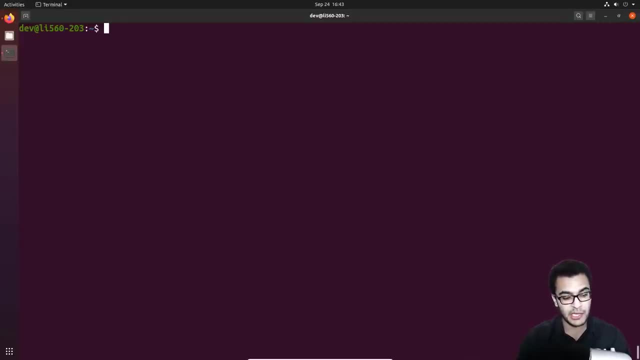 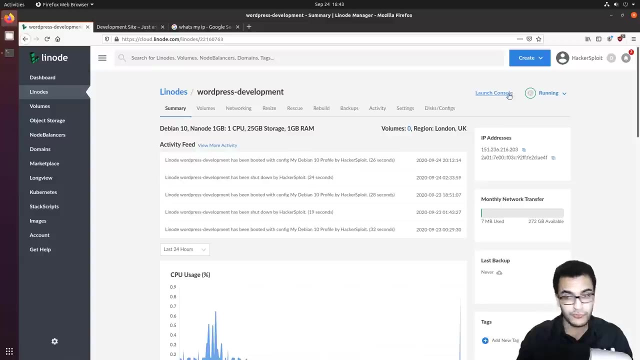 you want to make sure that you're not specifying a dynamic IP address that can then later lock you out If you're working with Linode or any other cloud provider. you also have the ability to get yourself out of trouble using the console here. 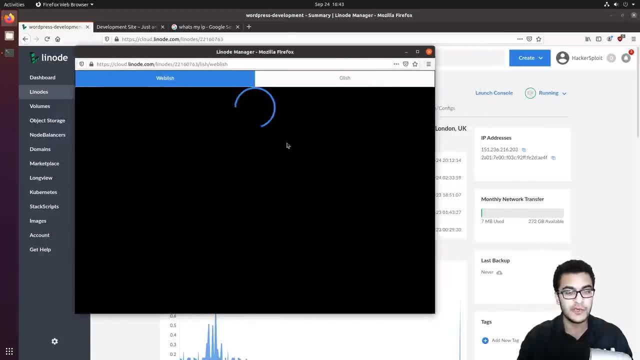 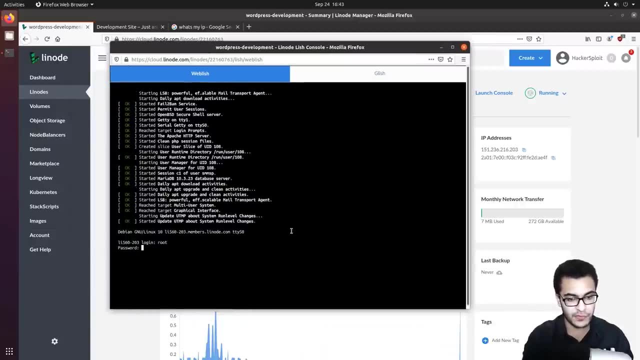 The console gives you a terminal within your browser So you can re establish access that way, and it does not use SSH by default, So you can actually just get access if I say root and here enter my password, which we had actually disabled, root through SSH. But you can see, I now 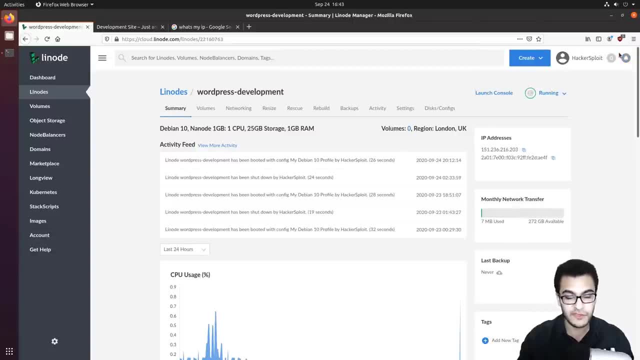 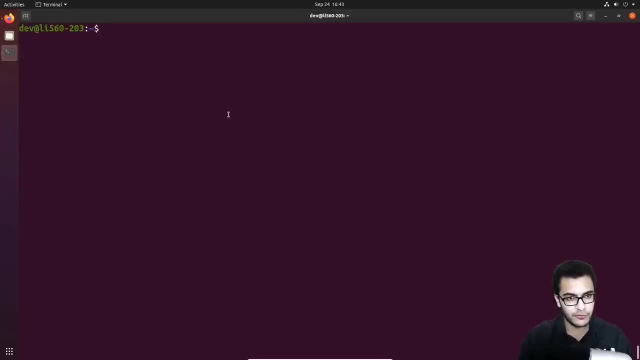 have access to the root account. So that's a great way to you know, save yourself or rescue yourself if you're ever in a situation where you've mucked up a firewall and you've locked yourself out. So it's always good to have that handy. So, deleting setting rules. 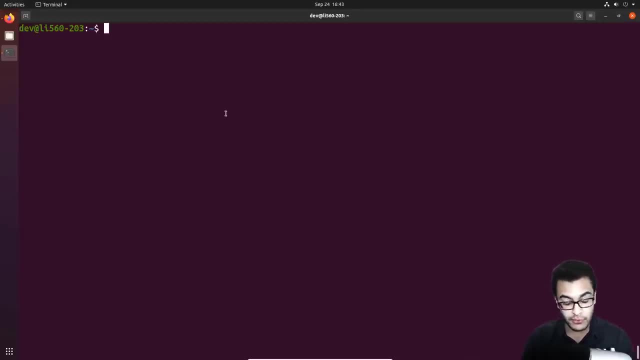 very, very simple. If you want to reset your, if you want to reset your FW, you can do that as well. So I can say sudo file. let me just list the status, or sudo ufw status. it's going to tell us. 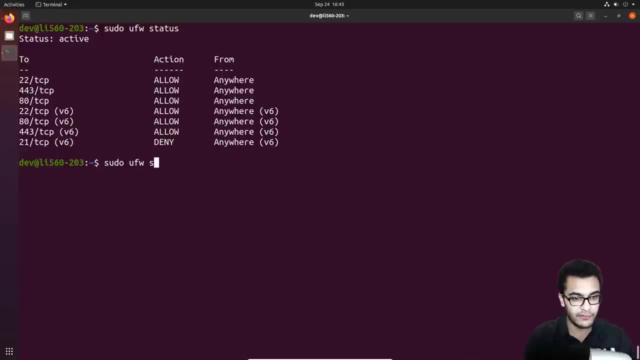 it's active, we can say sudo, sudo, ufw, reset. that's going to get rid of all your rules. So if you make, if you, if you make a mistake, you can reset all of those mistakes by just hitting enter, going to yes, and it's going to back up all of your rules. If we take a look at the status, 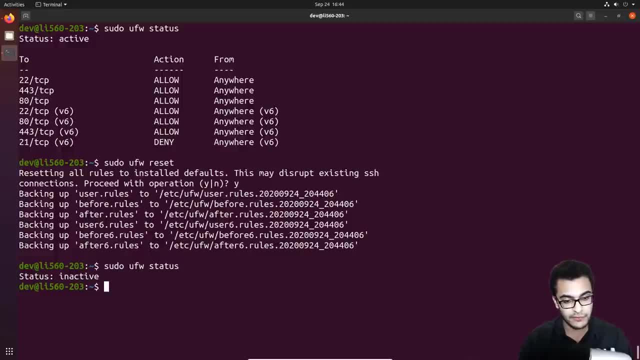 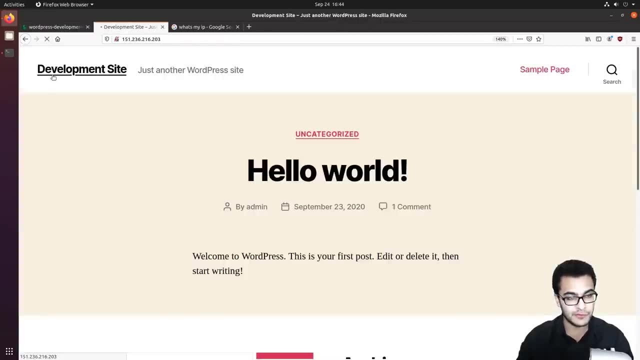 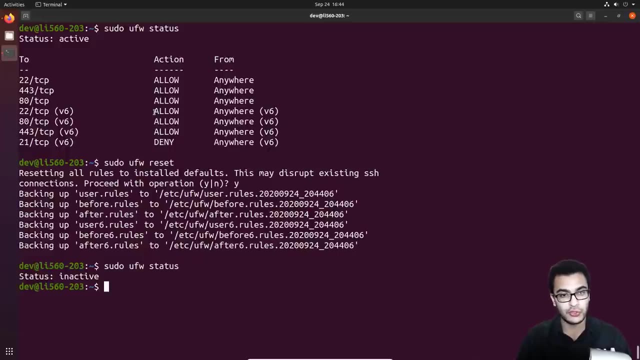 you can see it's still. it's going to tell us it's inactive when you, if you hit reset, is going to turn it off. And again, there we are. If we refresh this, we still have access to the site because the firewall is now enabled. Sorry, it's now disabled. So a few things I want to make clear. ensure that. 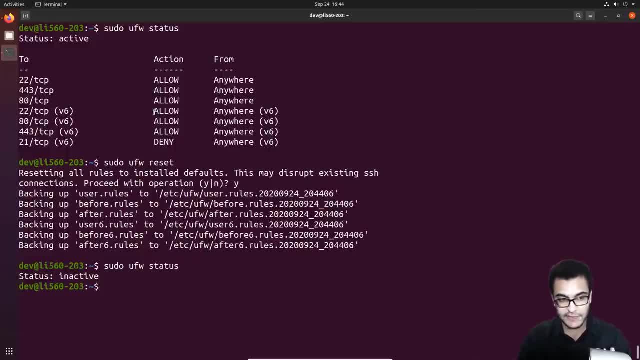 you set up your default policies first, then explicitly define the policies you want to allow in in terms of the connections you can also you can also define the ones you want to deny, then firewall, and then you can test it out that way. So ufw is very, very simple to understand. It's 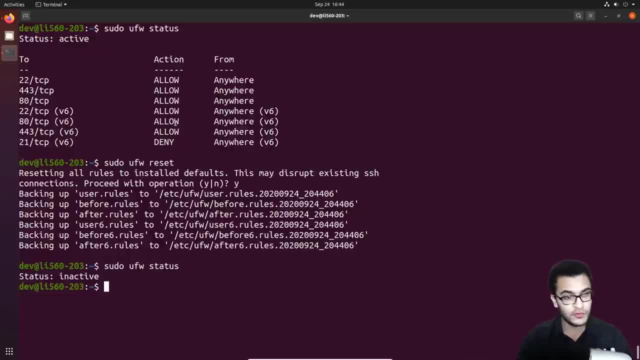 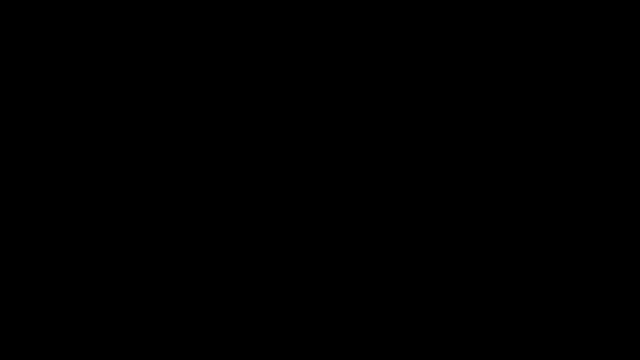 very intuitive, And it all revolves around what you want to do or how you want to configure your server. So that's going to be it for this video, And I'll be seeing you in the next video. I just want to take a moment to thank all our patreons at patreoncom forward slash. 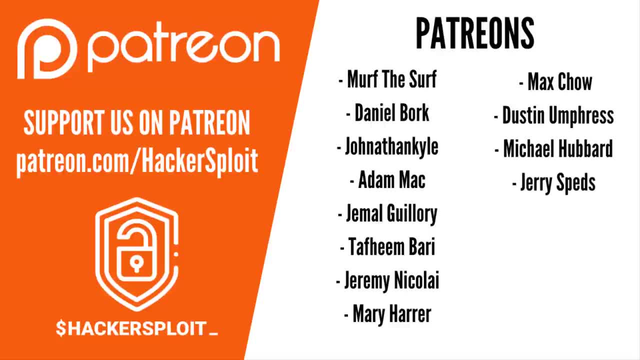 hackersploit. for all the support. your support and help is truly appreciated. You keep us making newer and fresher and better content, So I just want to say thank you very much. Thank you to all the patreons, So thank you Murph the Serf, Daniel Bork, Jonathan Kyle.